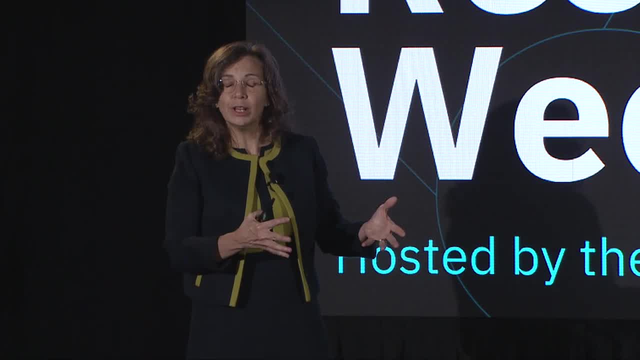 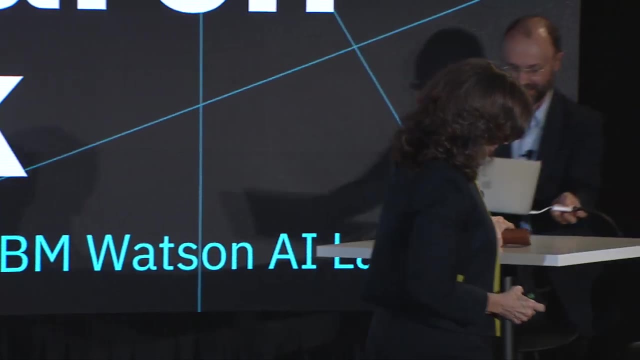 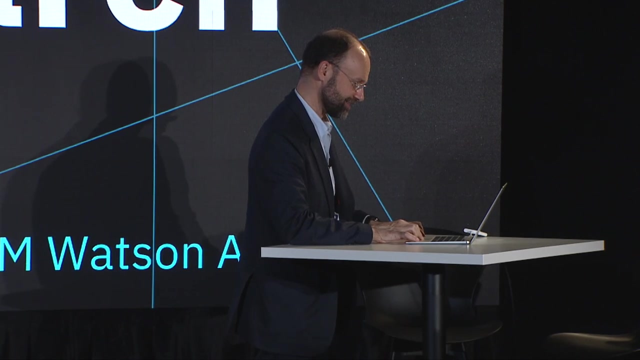 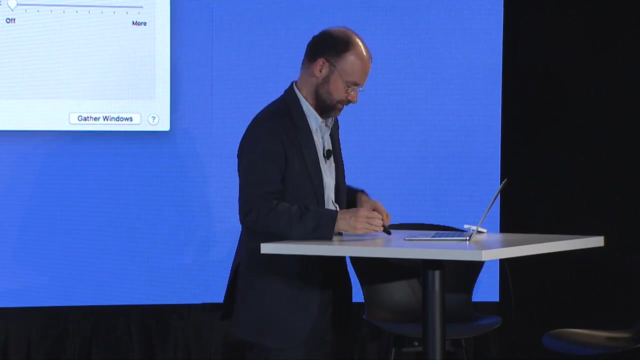 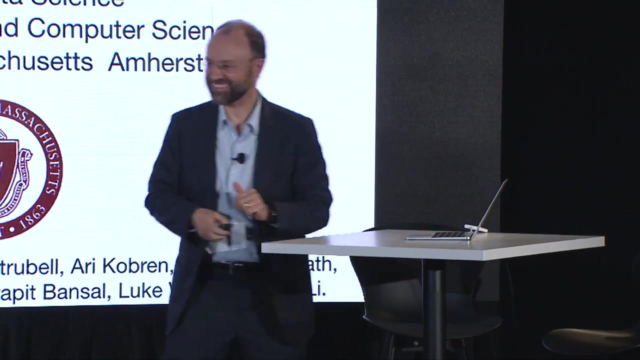 learn representations, to create learned representations from data and structured knowledge to support higher levels of reasoning, is truly at the forefront of AI research. So with that, please, please, welcome Andrew. Let's see, my screen didn't flash yet. Okay, good, All right. Thank you, Lisa. I really enjoyed Rob's talk so much. 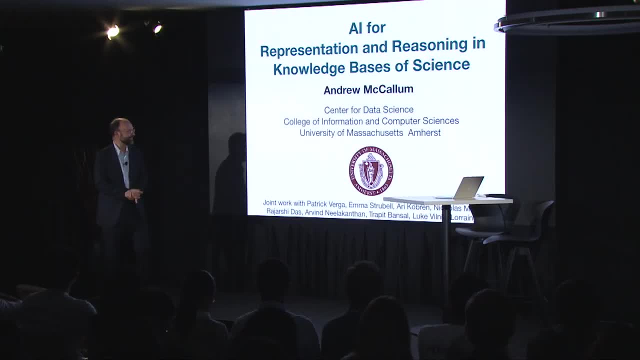 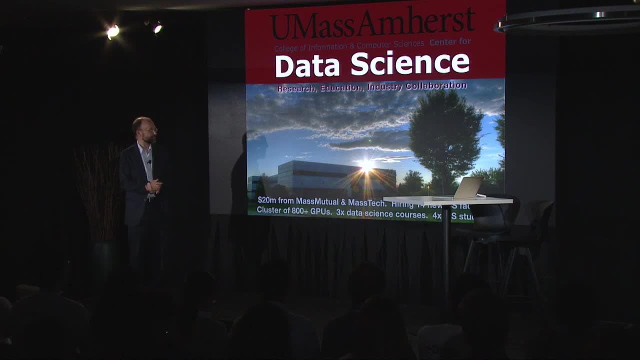 And I actually hope that I have some research that may help him more in the future. So I want to thank IBM for the invitation and for their support While I'm here. I also want to thank- sorry- the Center for Data Science on which I direct, which is not only enabling us to increase. 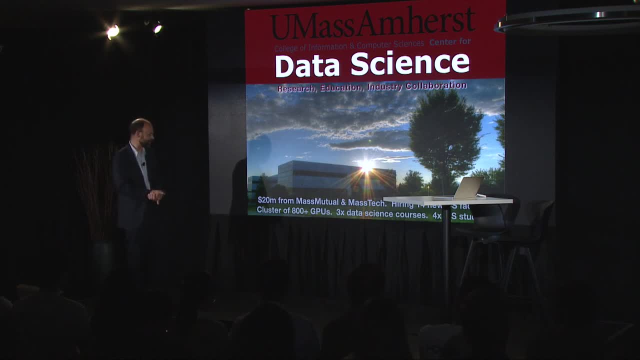 dramatically, say by 14 tenure track positions, the number of machine learning faculty we're hiring, but also enabled a lot of this research, because we used a large grant to gather a large computational cluster that has over 800 GPUs in it, which has just dramatically, you know. 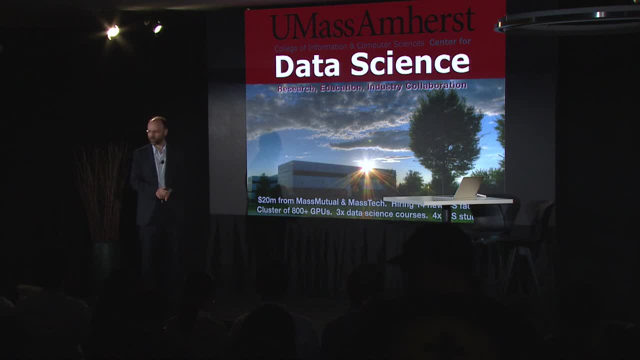 changed the way that we do research? I think it might be. I was talking with Yashua maybe a while ago, saying it might be the largest academic GPU installation anywhere in North America. Okay, And then for the industrial folks in the audience, I want to make sure that you know. 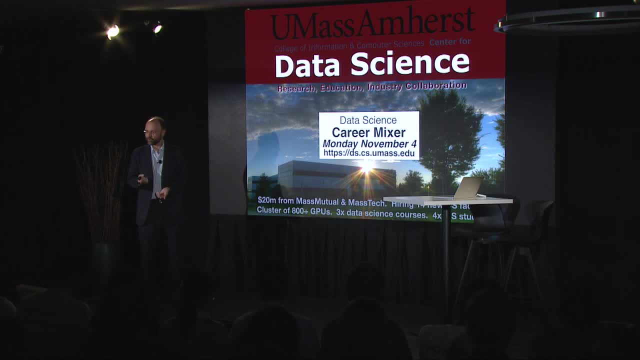 about, in about a month, a data science specific career fair that we'll be having, which a lot of our industrial partners have found a lot of good matches. It's mostly graduate students and they present posters as well. Okay, But we're here to talk about knowledge, representation and reasoning. 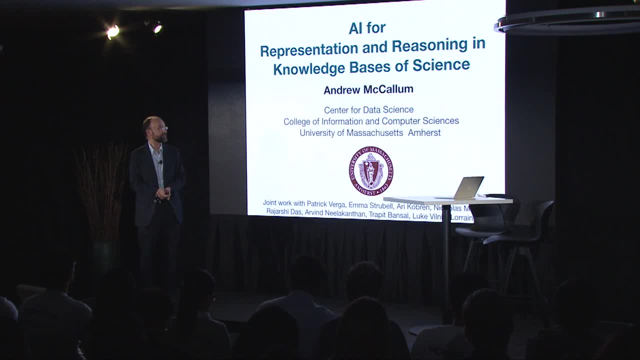 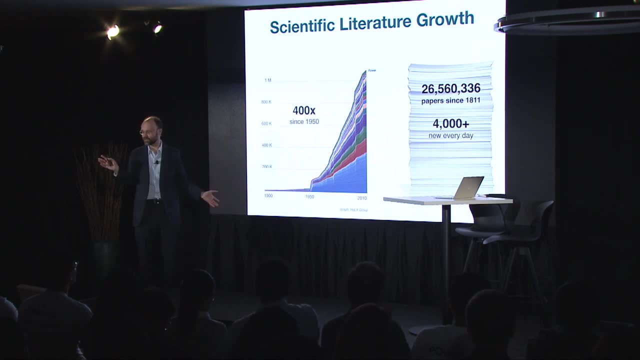 Which is one of the core aspects of artificial intelligence and, in particular, its application to science, And we really could use a lot of help, because the progress of science is accelerating rapidly and this means that the volume of publications is increasing as well. There was 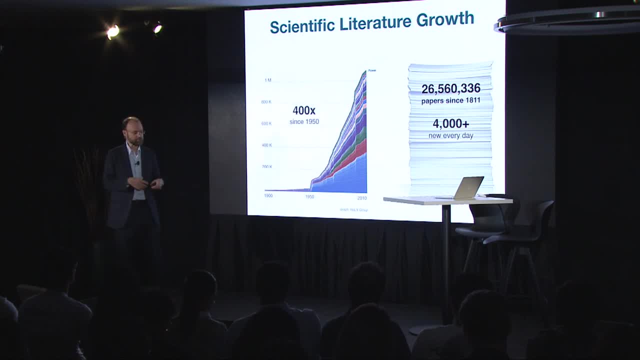 a survey recently of scientists, 85% of whom said I'm not able to keep up with all the research in my field, and I think the other 15% are lying And they need not just a search engine to help them find things. They're in the midst of designing experiments, deciding what directions to take in. 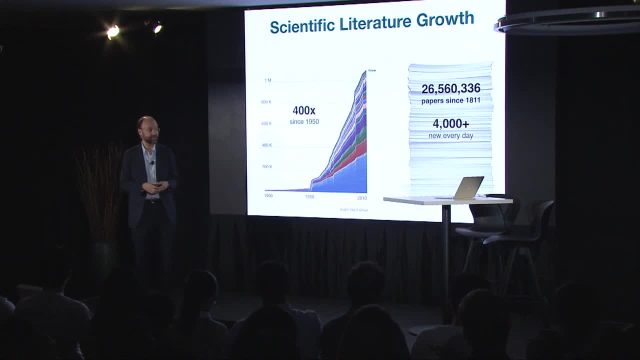 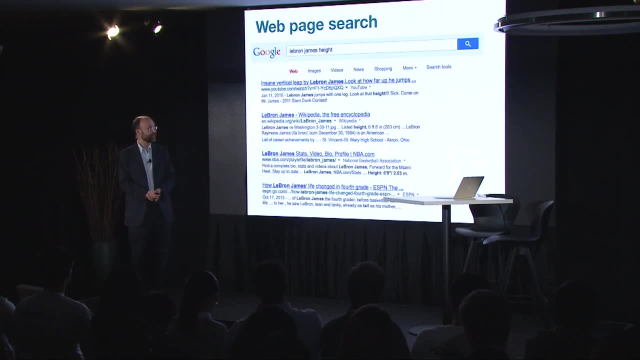 science. next, They really need navigational tools that will help them reason about science in order to help them accelerate their scientific progress. And there are many companies which, in their youth, started by focusing on keyword search, which, now that we're spending more time in front of, 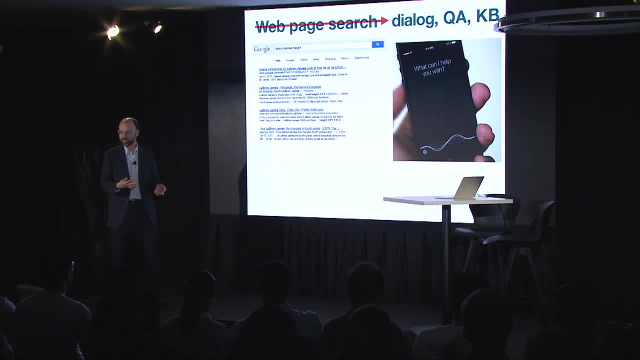 smaller screens are also thinking about dialogue systems, question answering, knowledge bases, a more structured view of the world in order to provide more succinct answers to questions, to provide ways to browse amongst entities through various types of relations. Types of relations here are shown in the bold text here. So these are types of relations, The catalog. 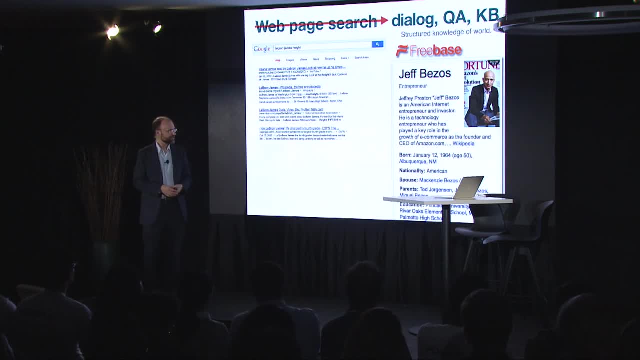 of the different types in this knowledge base was designed by humans to say: well, what are the kind of different semantics of relation types that we want to create? And they thought very hard about it. They created a large list, but in a sense it's not really large enough because, just as in web, 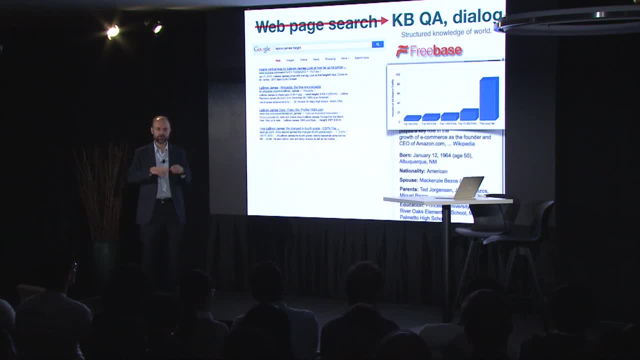 search the great diversity of things that people ask about. the majority of that mass is in the long tail of what people are asking about and the broad diversity. So, for example, if you want to know, well, who did Jeff Bezos criticize the Google Knowledge? 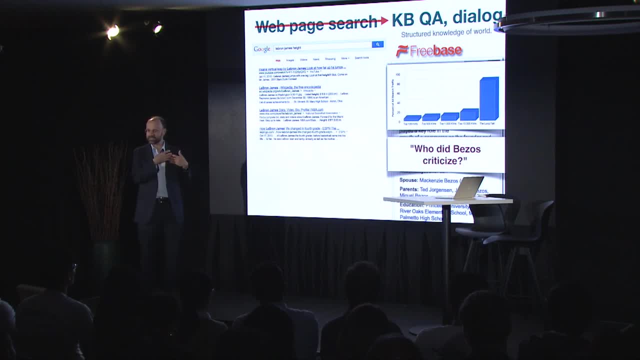 Graph or Freebase or many others can't tell you because they didn't create this relation in their knowledge base. So what we're really interested in is a knowledge base with an open schema, sort of like keyword search, where you could ask about absolutely anything but at the same time that 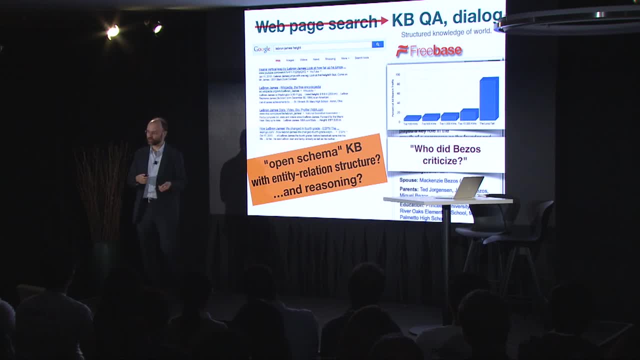 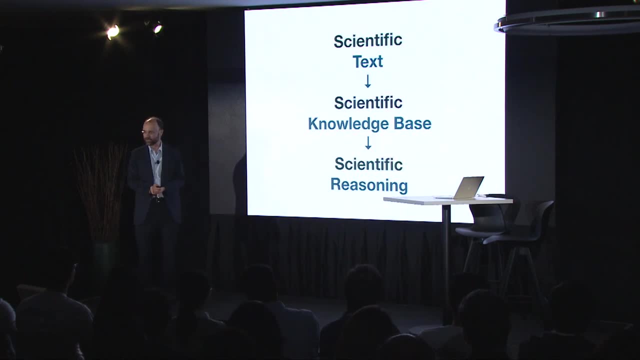 has a structure of entities and relations, and one that will support reasoning, And that's really what this talk is going to be about. So we're going to talk about going from text to knowledge bases, to reasoning, and especially doing this in the context of science, And this is an area which I've had interest for. 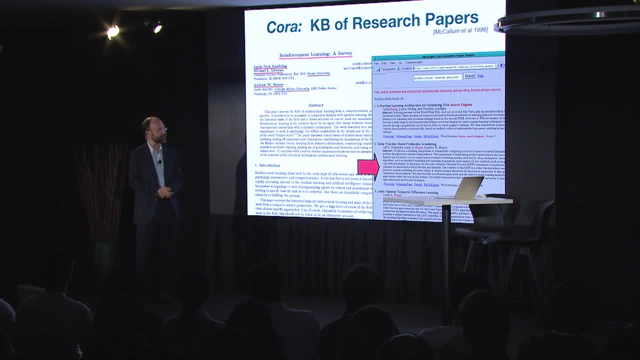 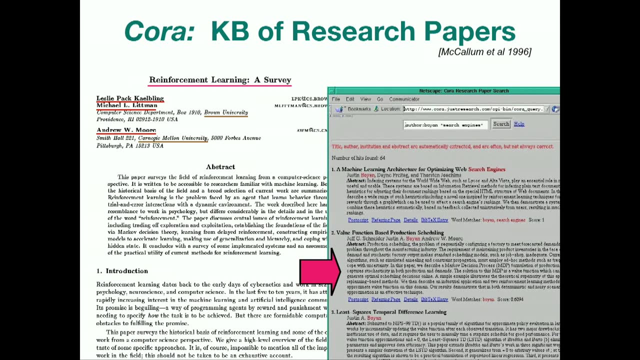 quite some time, about a decade before Google Scholar existed. Some colleagues and I at Carnegie Mellon built a system that had many of the similar features. You can tell how old this is by looking at the header in the web browser there. When I arrived at UMass, we built a more modern system. 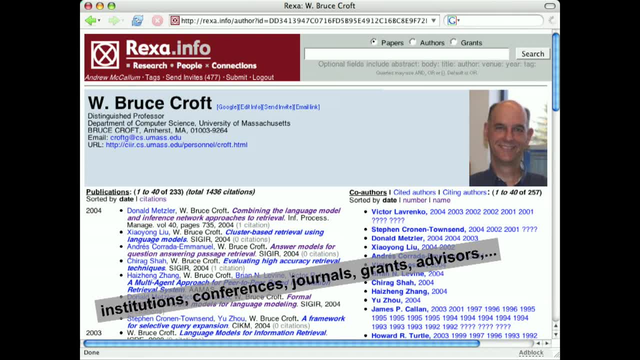 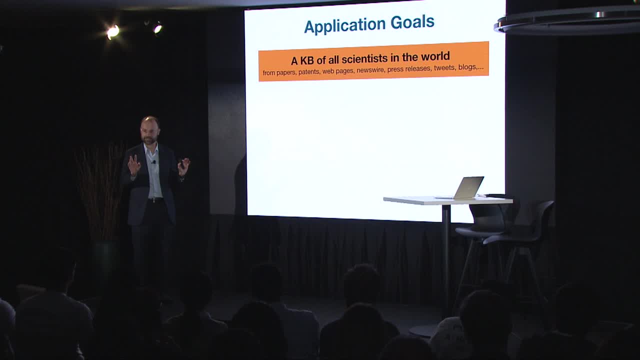 that knew not just about people and papers, but institutions, conferences, journals, grants, advisors and the rest. And really now we're working on multiple thrusts, one of which is to build a knowledge base of all scientists in the world and their expertise. 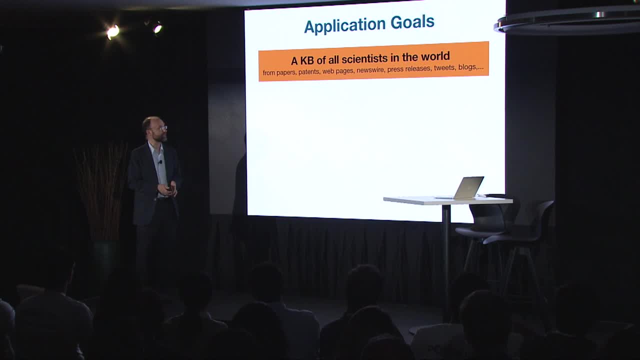 and their career path history by gathering information from many places, as well as to build a knowledge base of scientific entities and relations, things like materials, equipment, organisms, processes, tasks, methods- many of the things that we heard about from Rob, And so we'd. 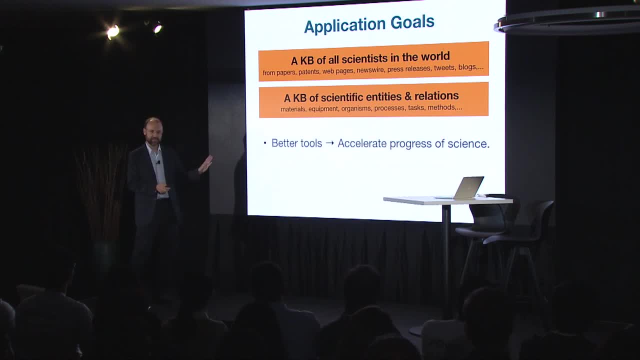 like to do this for the obvious reasons. Just as a brief aside, I'm also very interested in revolutionizing scientific peer review. I think the time it's high time that this happened. The way that scientific workflows for review happen right now were designed in the times when we were 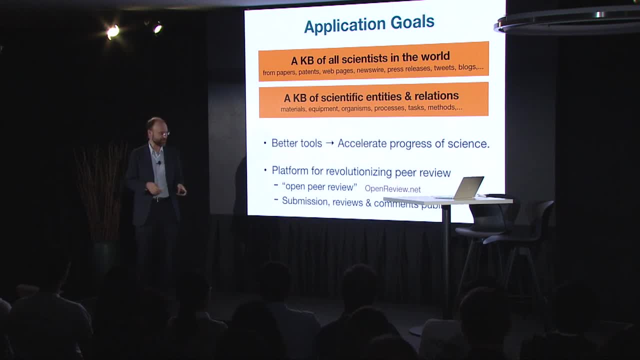 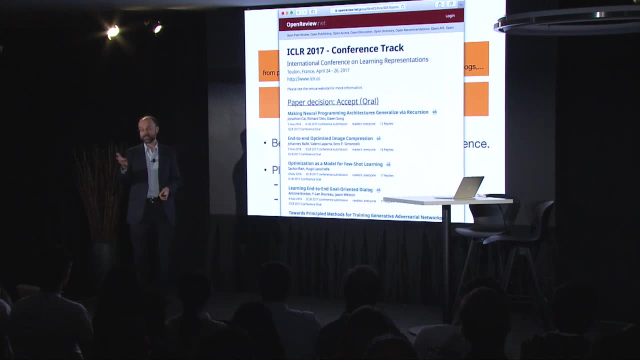 printing research on paper and sending it through the post, and we have much better methods of doing this now. We've built a system called openreviewnet that was actually but just served the deadline for the iClear conference just last week, accepted about a thousand and a half papers in just 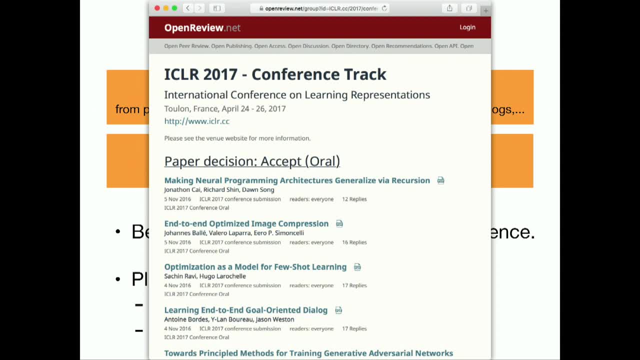 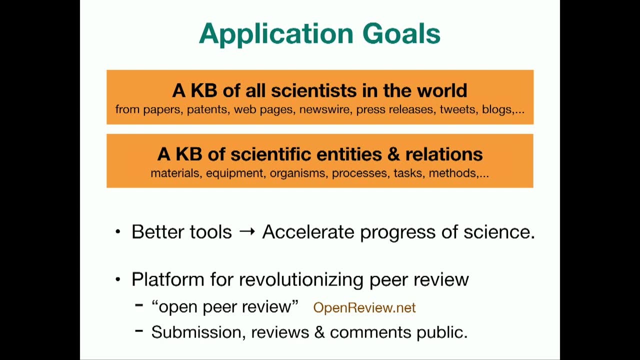 a few hours. It's being used by about 20 different venues. now We're in discussions with ICML, CVPR and others, And if afterwards you want to talk about that, I would love to tell you more about that, All right, But what I mostly want to talk about 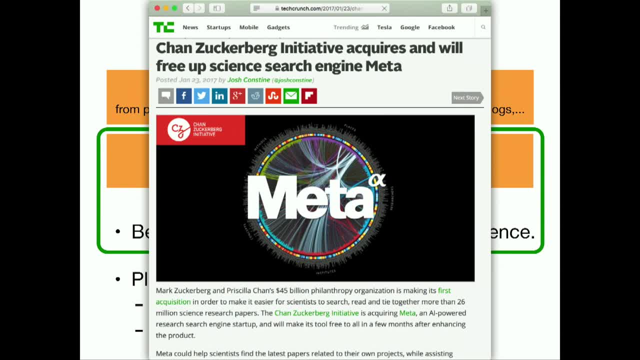 here is that we're going to be talking about a lot of different things. We're going to be talking about the scientific entities. So I have been working with a Canadian startup company that shared many of the same goals that was acquired by the Chan Zuckerberg initiative. This is not. 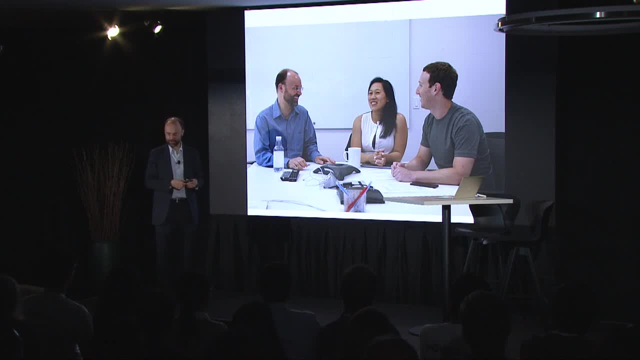 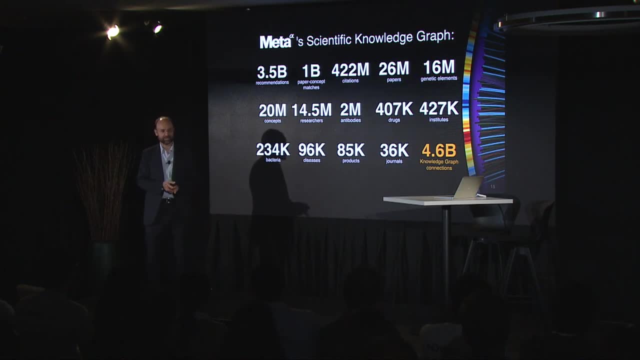 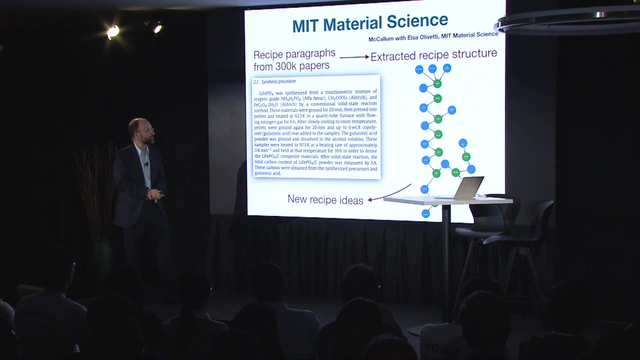 Facebook, but the philanthropic arm of where Zuckerberg has pledged to give away the vast majority of his wealth, And they have an extremely large knowledge base based on scientific entities. If we just take one column here, so like 26 million papers, over 400,000 drugs, 36,000 journals- many of these connected in the web, And we've been working. 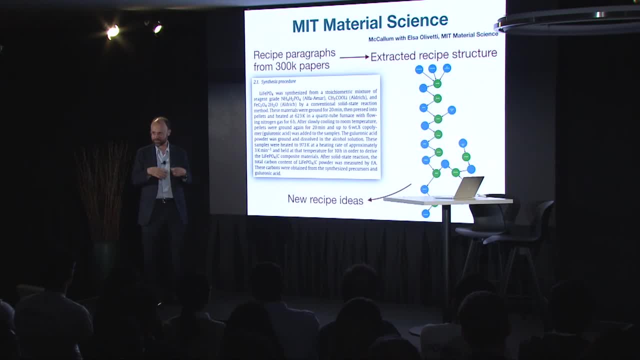 together to both enlarge that knowledge base and to do reasoning about it with techniques that I'll describe in a minute. We've also been collaborating with folks right here at MIT in material science to gather hundreds of thousands of research papers from material science, automatically finding the section where they describe the recipe- and it really does look like a recipe. 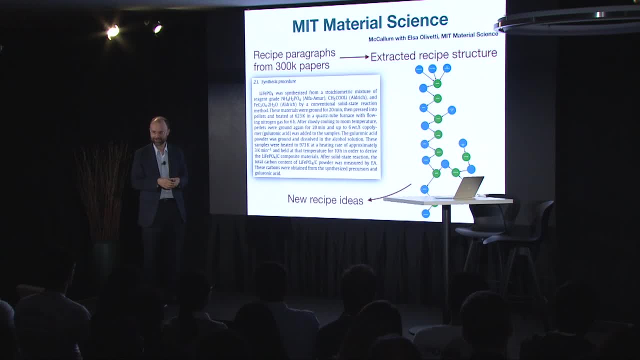 for cooking up a brand new batch of, say, car battery materials of the future, extracting that recipe as a structured graph and then doing analysis on a large collection of recipes to understand the relations between the recipes and the properties of the materials that result, to suggest brand new recipes that have 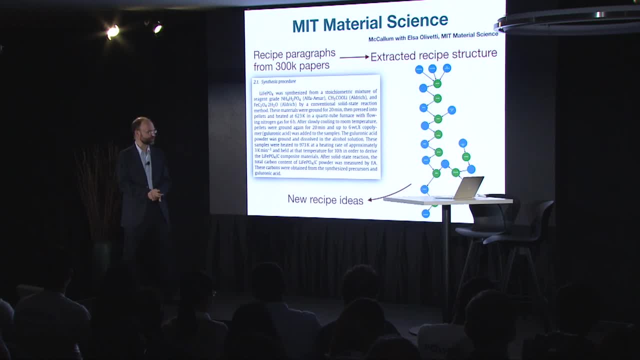 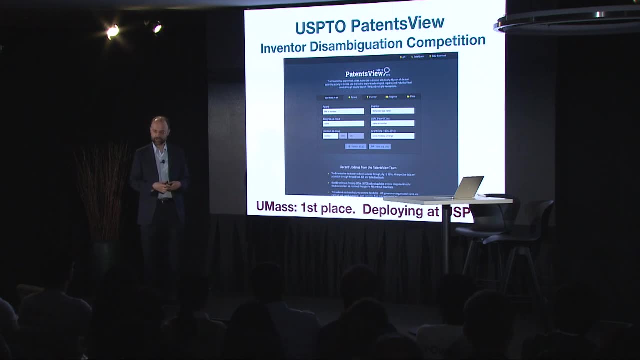 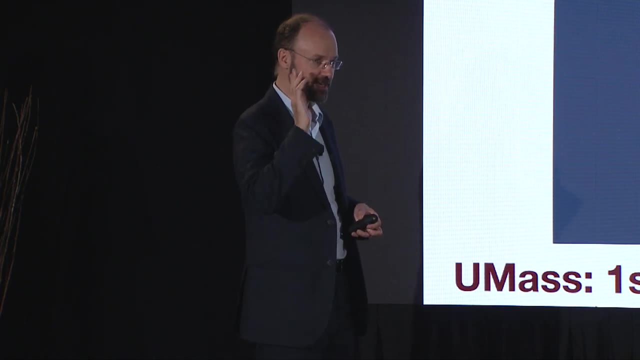 never been tried before. that might help us address global warming issues a little bit quicker. We also have been working with the US Patent Office to design new, more accurate methods of resolving authors of both patents and research papers, And this is work by Nick Monath, who is here with us today and has a poster here today. 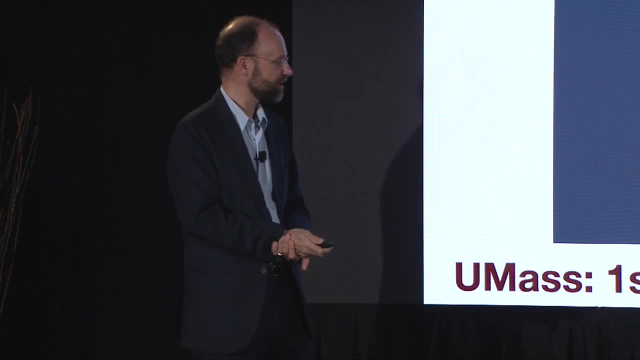 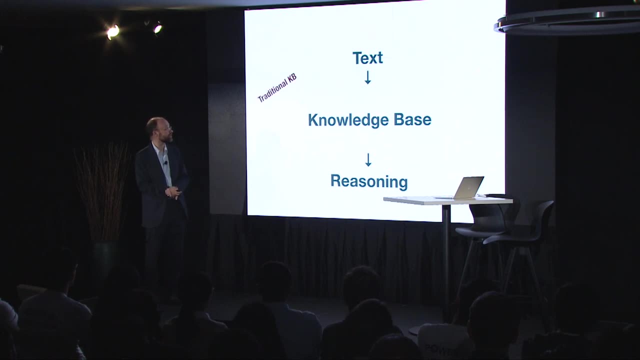 and his work is now being deployed as part of the US Patent Office workflow. Okay, but those are just a few examples. Mostly, I want to talk about the technology for how this happens, And in a traditional knowledge base, the knowledge base consists of entities and relations. 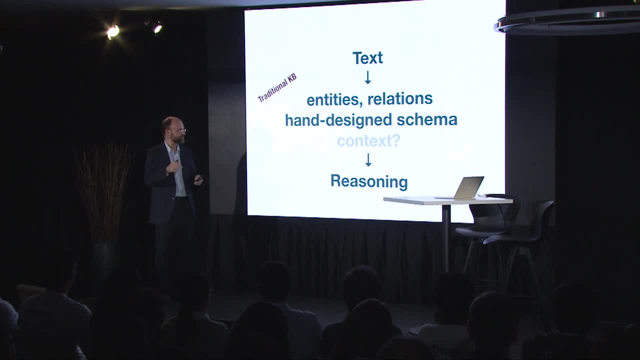 and, as I was describing before, some hand-designed schema for entity types and relation types, And this is exactly what's in Freebase and various other traditional knowledge bases, as well as in medical knowledge bases like SNOMED and many others. We're going to be talking, instead, about replacing the hand-designed schema with something we 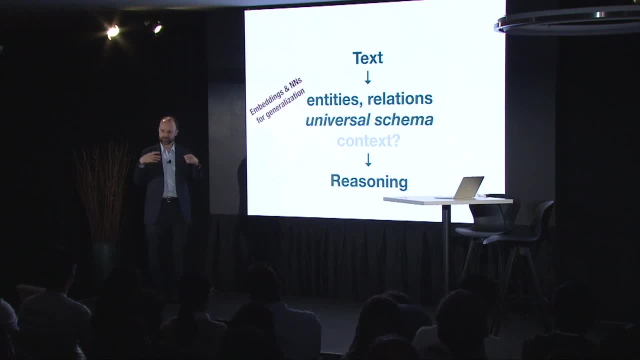 call universal schema, which I'll describe in a moment- which is based on vector embeddings and deep learning in order to gain some generalization capabilities, and also using textual content and looking quite a bit at the degree to which that raw text itself can serve as a knowledge. 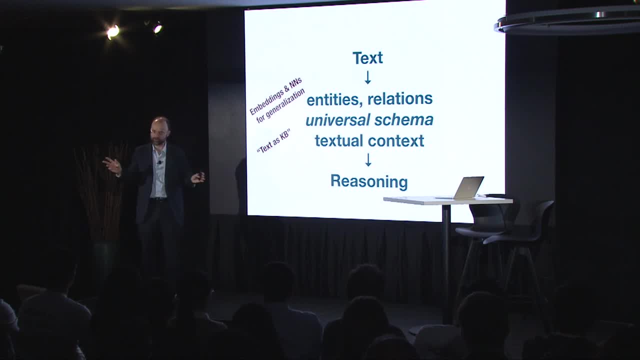 base, But we also want to build a graph at the same time in order to be able to navigate through them and this landscape of sort of smooth landscape of working with raw text versus a very structured content. But today, the two technical things I want to focus on most are some work on chains of 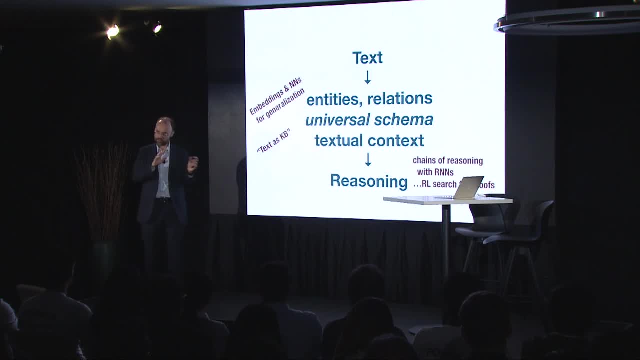 reasoning with recurrent neural networks in a way that really bridges symbolic AI and vector-based or neural network AI, And we're going to talk about using reinforcement learning to search for proofs in this space, And I also want to talk a little bit about some of the things that we're going to be. 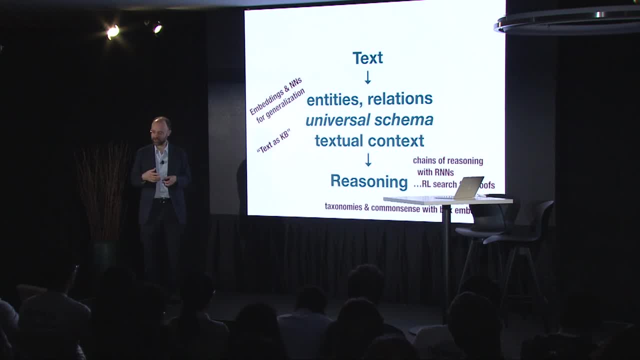 talking about. But first I just want to talk about efficient methods of representing taxonomies and common sense using a new technology we've been working on recently that we call box embeddings. Okay, let's first start with an introduction. So to build a knowledge base, we usually start with a raw set of text. 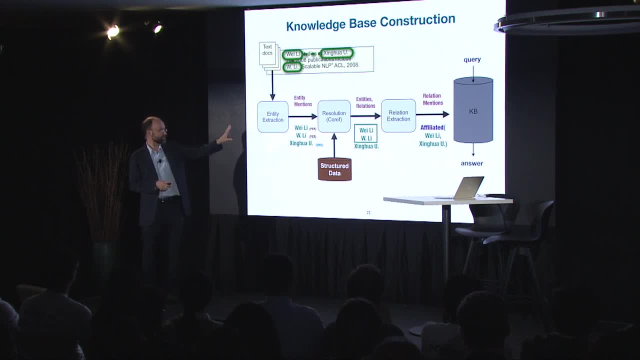 From there we need to find some entities. we need to resolve multiple occurrences of those in both unstructured and structured sources. do relation extraction on top of those, put those into a knowledge base which then, given a query, can hopefully answer some questions. 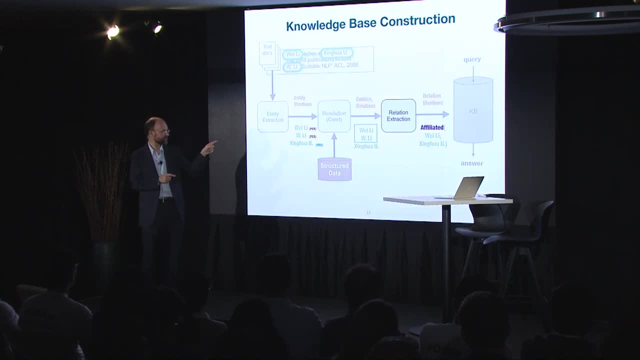 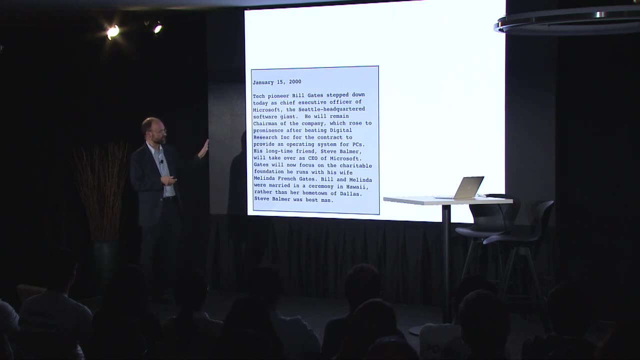 And what I want to focus on most here are these types of data, the different types of entities, the different types of relations and where they come from. So let's first step back a little bit. We've given some raw text And, with apologies, this text does not actually have to do with science, because maybe many 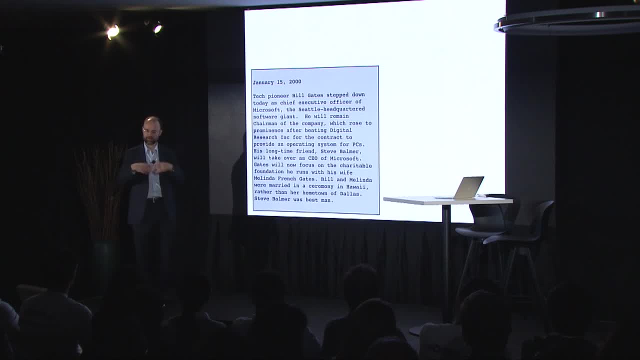 of us aren't bench scientists and I want to work with data and make a presentation that we can all understand intuitively, but I'm going to rely on your imagination to understand how this would apply to science. So we're given some raw text. 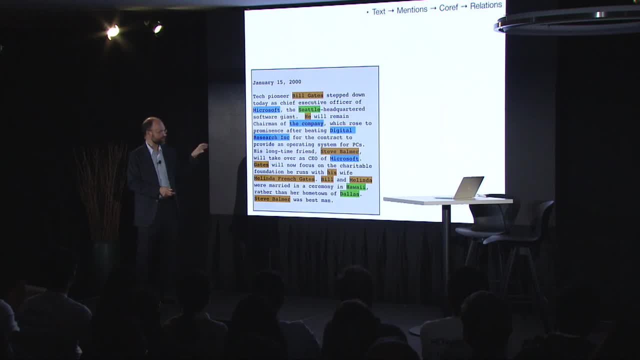 From that we extract some data. Okay, So we have the names of some entities and we resolve them, knowing when Bill Gates and Gates are referring to the same person. From that we can build a graph of these entities and the sentences in which they co-occur. 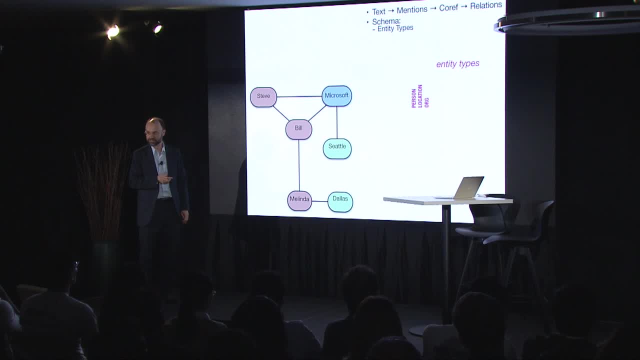 But to really understand what's going on here, we'd like to know well what are the types of the entities appearing in the nodes of these graphs And what are the types of the relations appearing on the edges between them. So let's focus on the entity type for a moment here. 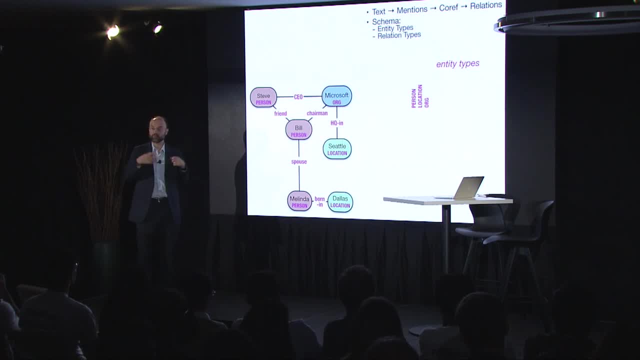 So here are some types that we may have had in our head that we thought would be important for our application, And we're going to end up importing data from multiple sources to help augment our graph, But that data will come from some other source and some other person to design some other. 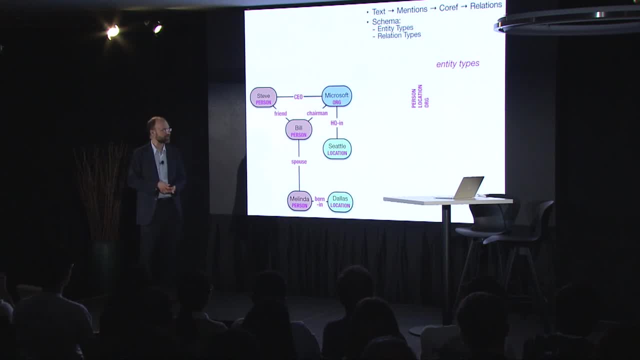 schema that's almost surely not going to match our schema of different entity types. They'll just be different And unfortunately it's usually not so easy just to map them deterministically one on top of the other rather than overlapping by containment or by exact implicature. 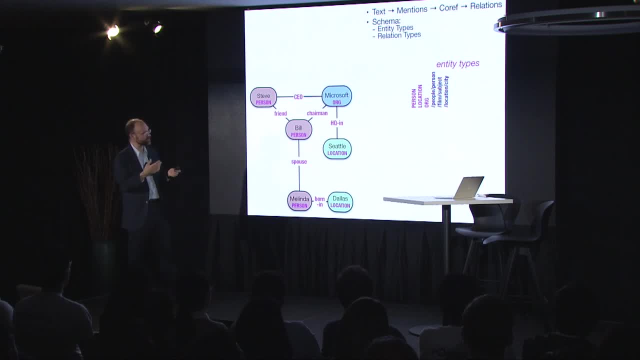 So often these concepts overlap, sort of partially, Like this. So like a film subject- which is one of the columns here- is often a person, but sometimes it's a dog or some other creature, And so they overlap partially. So rather than trying to map all of our semantics onto a single schema to rule them all in, 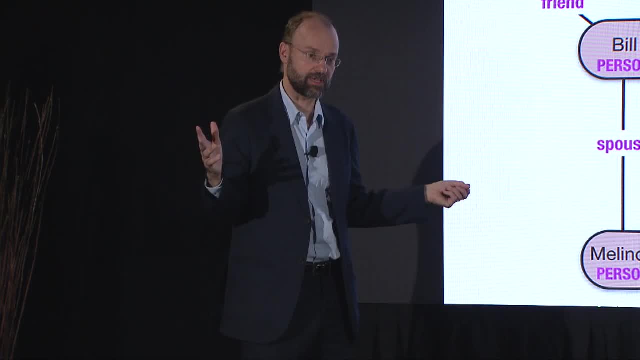 universal schema. we're going to keep around all of our input schema, not try to cram all of our semantics into one box. embrace the full diversity of it all and then learn the basics of it all, Something about how these different schemas have some mutual implicature among them. 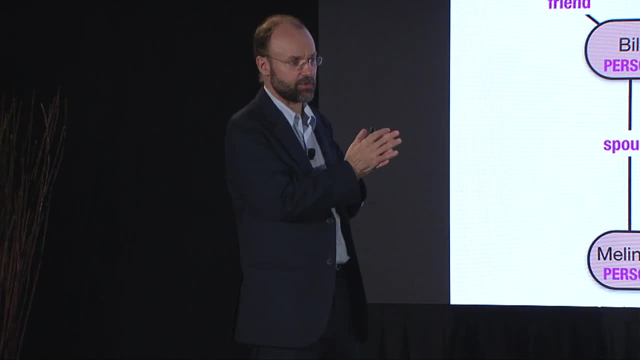 And furthermore. so actually I'm only going to show a few examples here, but you can imagine actually we might be working with 20 or 100 different databases, all with their own different schema, And each one may have thousands of different schema items in them. 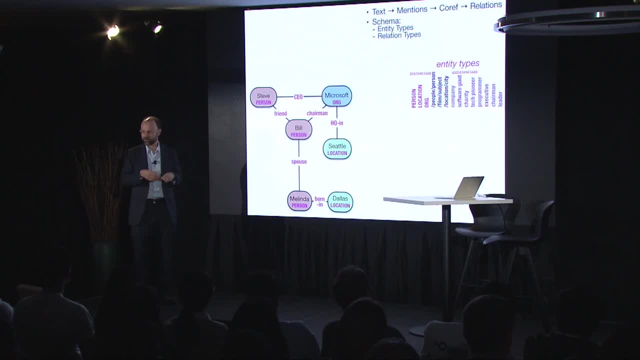 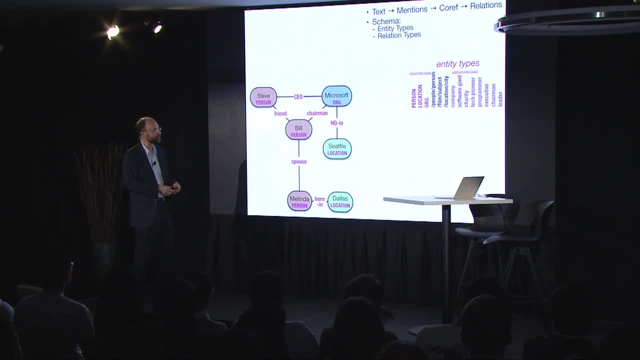 So an additional tens of thousands or hundreds of thousands of schema items might come from here as well. So we're going to keep these all around, and this is what I mean by universal schema. So it's our job to take some input, context and to classify the appearance of this entity. 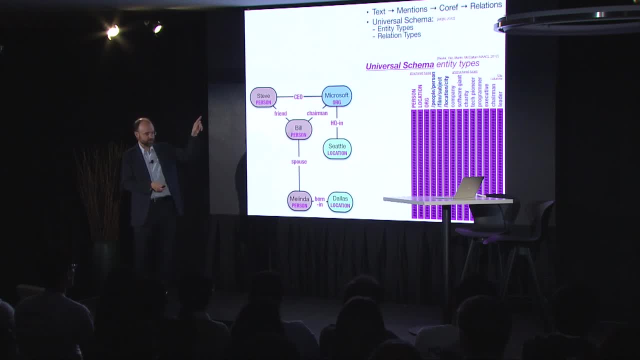 as to which entity type it is, And rather than having a set of parameters shown as a purple vector here in the original raw feature space, we're going to learn them in some compacted latent space I think about. it's like a word embedding in, say, 100 dimensional, 200 dimensional. 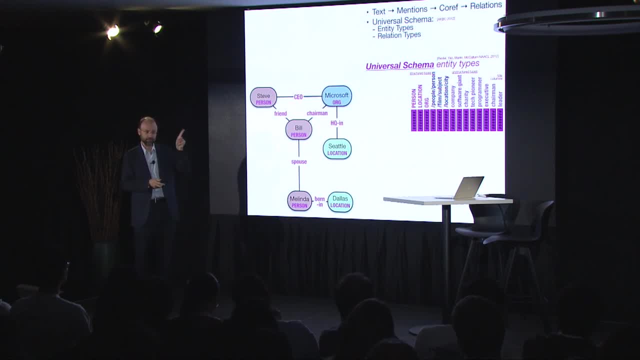 space where the individual dimensions don't really have any meaning here. But we're going to learn these vector embeddings so that types that have similar meaning appear near each other in this vector space And the entities we want to classify will get embedded in the same space. 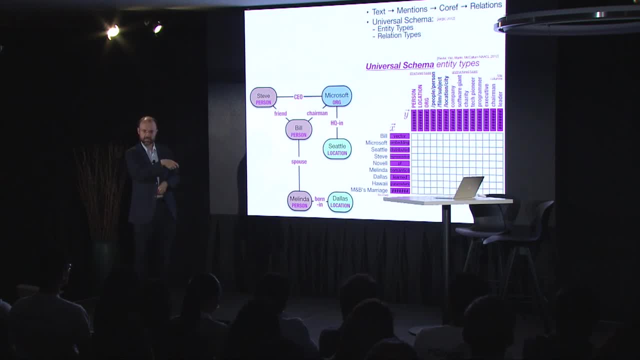 And I can make a prediction about whether some entity is an instance of some type by doing a dot product between these entities. So at training time I'll observe from my raw data some of these entities and which types they belong to, And it's my job for the sake of. 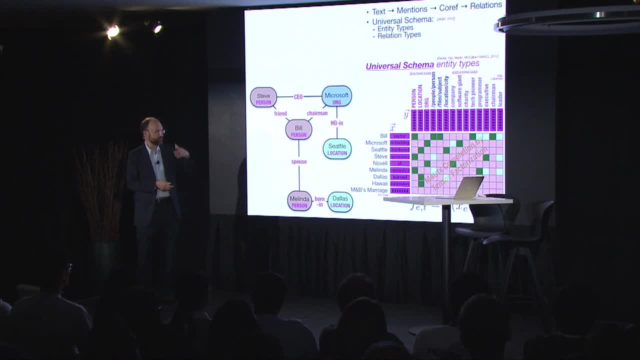 The full completion to do matrix completion to fill in some of those missing ones, so that, even though I didn't observe originally that Bill was an executive, I can predict nonetheless he is an executive from the co-occurrence of other types that I did observe him for. 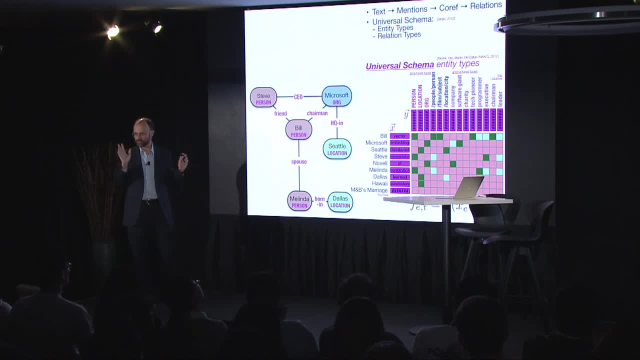 And this kind of matrix completion is exactly what Netflix uses to recommend movies to you, given the partially completed matrix of what you and others have told it about what movies you'd like. The same thing can be done for relation types in which we have different types of relations. 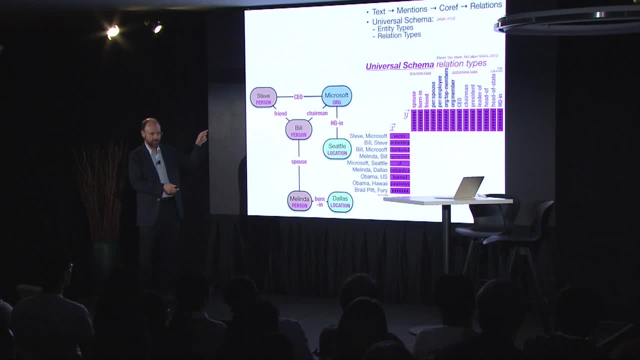 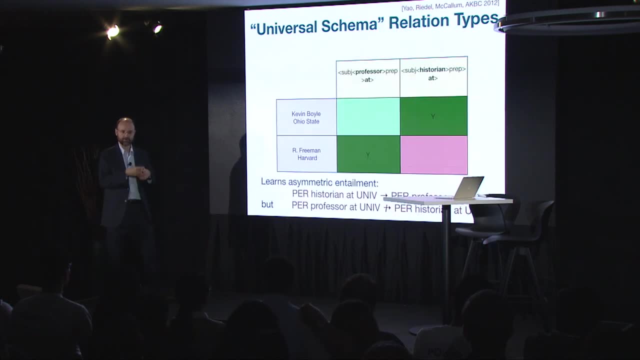 in the columns, from both multiple structured sources and from text, And then entity pairs, And again we can do matrix completion to predict new relation types, And just to give you some visceral sense of how this works, for example, this comes from some real data that we ran on. 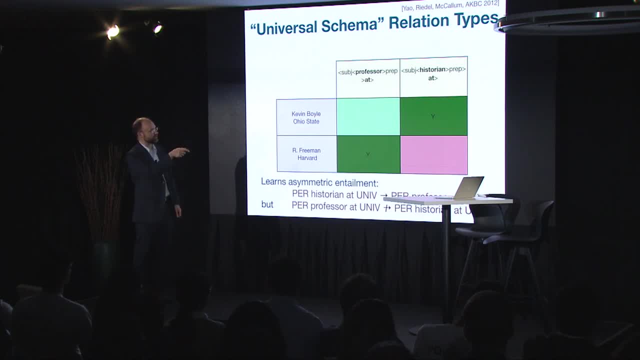 The system observed that Kevin Boyle was a historian at Ohio State and from that we predicted that he's a professor at Ohio State. And yet, in a demonstration of the model's ability to represent asymmetries, when we observed that Freeman is a professor at Harvard, we didn't necessarily infer that he's a historian. 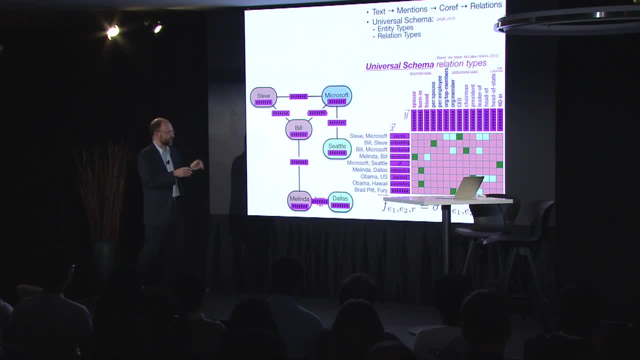 All right. So here we end up with a knowledge base, that's, a graph of entities and relations in which, rather than having symbols sitting on the nodes and edges of the graph to communicate the semantics of what we really mean here, we have these vectors instead. 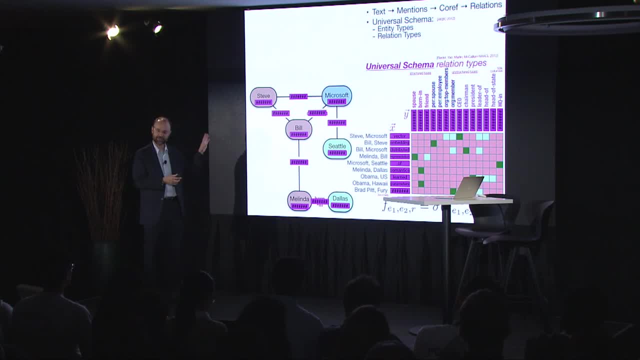 Vectors, representing a broad diversity of different kinds of semantics, And I find this really interesting. I think about mixing vector representations and graph representations And, furthermore, thinking about how you know, philosophy and computer science and mathematics has spent decades studying what it means to do logical reasoning on symbols, And here we're about to ask ourselves: 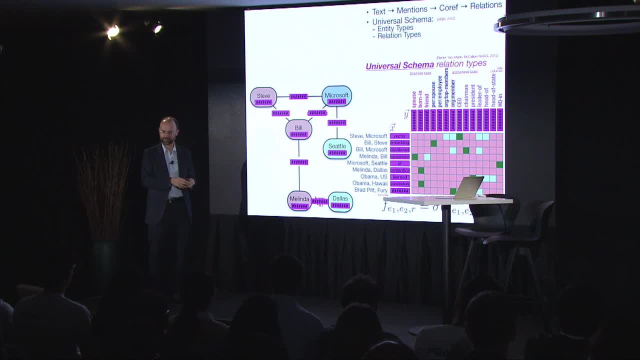 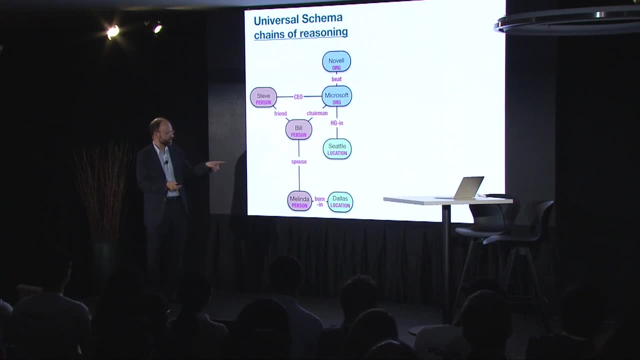 well, what does it mean to do logical reasoning on vectors instead of symbols? Because reasoning is exactly what we'd like to do in this kind of knowledge graph. So here's what I mean by this. Let's say that someone asks about the nature of the relationship between Melinda and Seattle. 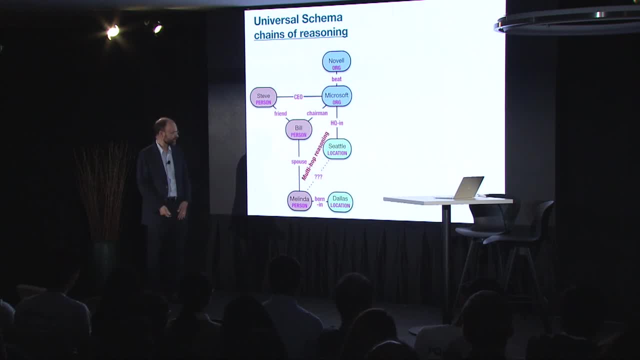 Well, we didn't observe any raw evidence of what that relationship is, but there is some other evidence in the graph that we can form through some chains of reasoning right That literally consists of a chain through the graph, some path of the graph right. Melinda is married to Bill. 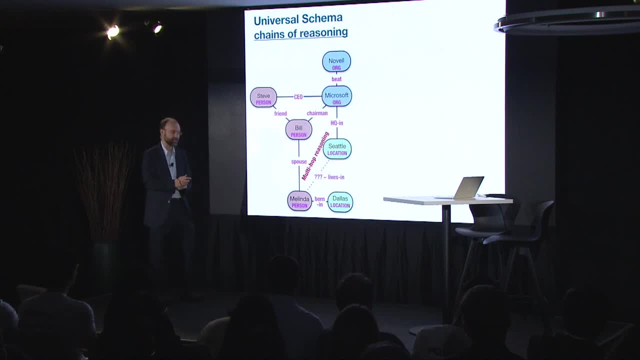 who's chairman of Microsoft headquartered in Seattle, and perhaps we can use that as evidence with some probability that perhaps Melinda lives in Seattle. And then traditionally I would write this down as a symbolic rule, right, If A is the spouse of B. 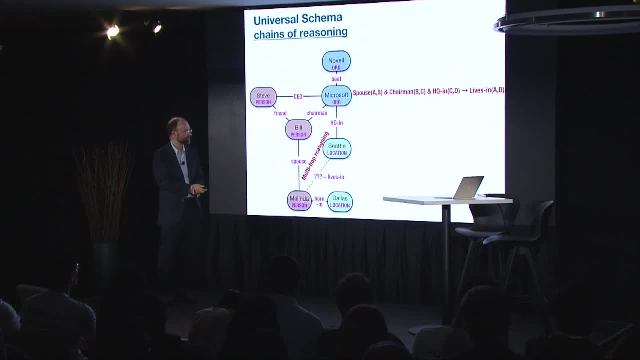 and B is the chairman of C and so on. then A lives in D. But what if, in the data that we're asking about in the graph, there's no evidence that we can form through some chains of reasoning? Instead of chairman, it was CEO. Okay, well, we need another rule for that. Or what if it was COO? 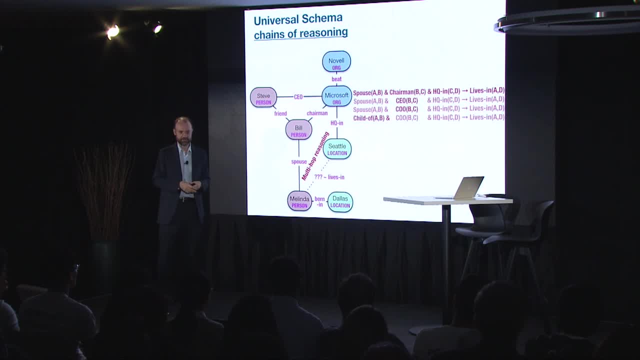 instead. Okay, well, we need another rule for that. Or what if it's child of instead of spouse of? Well, now we need a combinatorial combination of a number of different rules to cover all these cases, and hence the difficulty of symbolic AI. But here we have vectors in this graph instead. 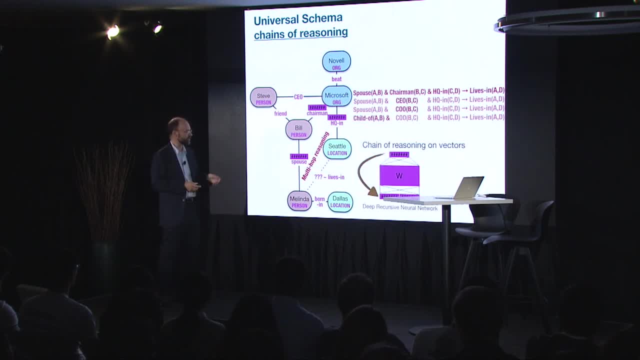 which are exactly designed to help us generalize, And so we've been working with methods that consume arbitrary length chains through a graph like this: At each stage pumping that vector into a recurrent neural network that consumes the new piece of context in the chain and, at each stage, outputs a new vector that represents the nature of the semantics. 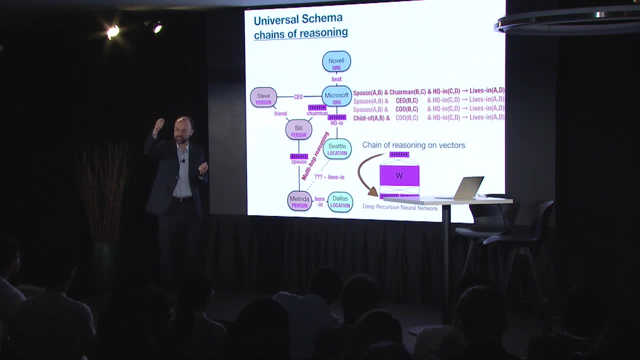 between the two nodes. that are the endpoints so far, And when I add another link, then I now compose my semantics further to represent the nature of the relationship between them. And indeed, when we train on data and pass a path like this into our network, it does predict. 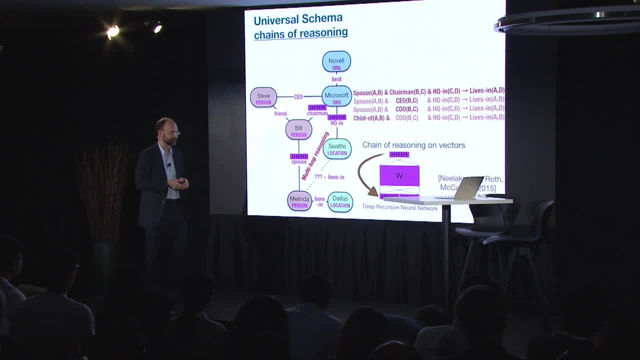 or the vector it produces is very close to the vector for the symbol it lives in. So the neural network has learned how to do logical reasoning in this method that goes beyond symbols, that learns to generalize. So we've run this on a moderate amount of data from Freebase and from text. 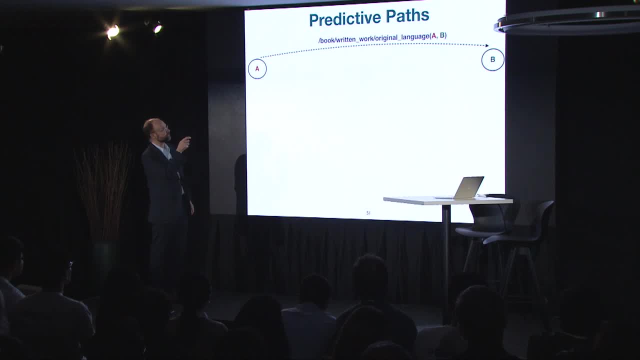 and to give you a sense of the kind of paths that it can learn. So here we're, predicting the relation of book and the original language in which the book was written. And here's the path that the method discovers: It goes from a book to some other book that's previous in a series of books. 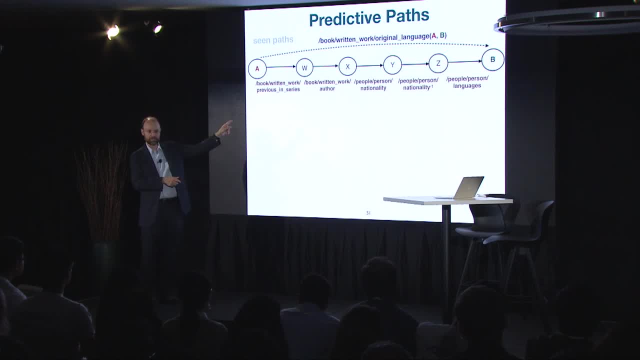 Think, like Harry Potter, To the author of that book, to the nationality of that author, to somebody else who shares the same nationality, to what language do they speak? And that seems like a reasonable chain to have some level of inference about what language we. 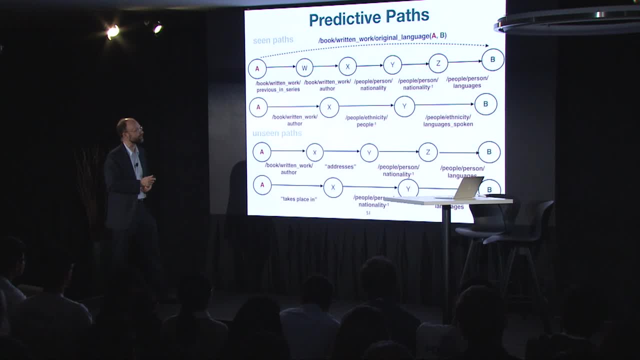 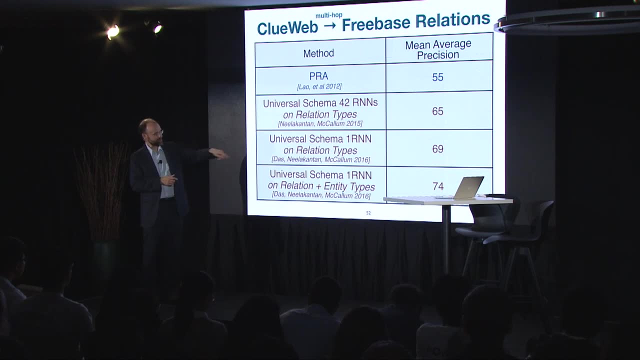 think the book was originally written in, And there are many other examples I'm not going to take the time to show you All right. So for some of you in the audience, you've seen some of this context before, Sorry. let me say first that, as is typical in research, 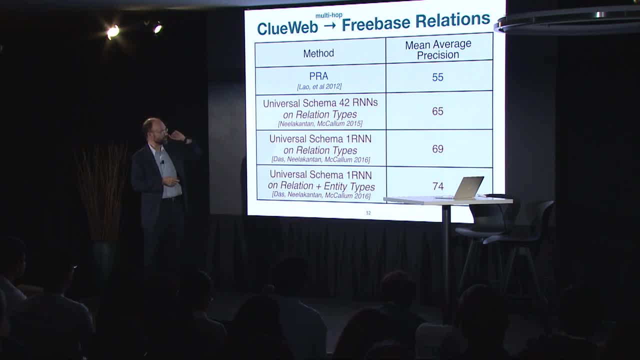 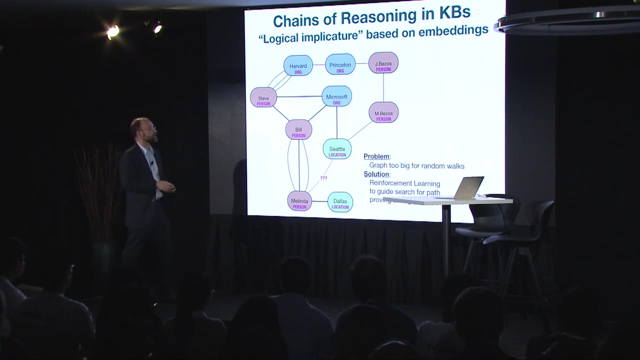 in comparison with an older symbolic method that came out of Carnegie Mellon in 2012,. over time, we are gradually making accuracy improvements And I think we're on our way towards a system that would be usable for deployment. But some newer work that I want to describe today are addressing: 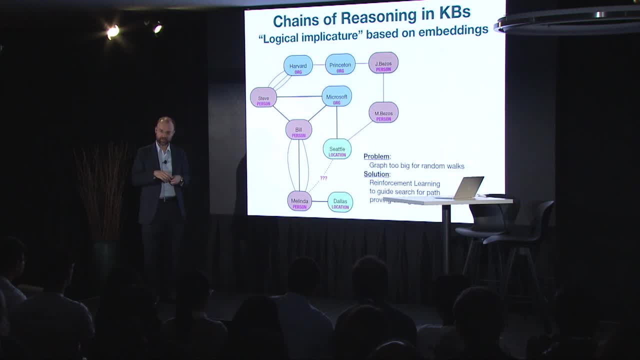 the situation that occurs in really large graphs, in which it takes some careful effort in order to find the chain. that gives you a proof for the answer to our question. So there's some paths That might be relevant to the question that we have, but there are many other paths. 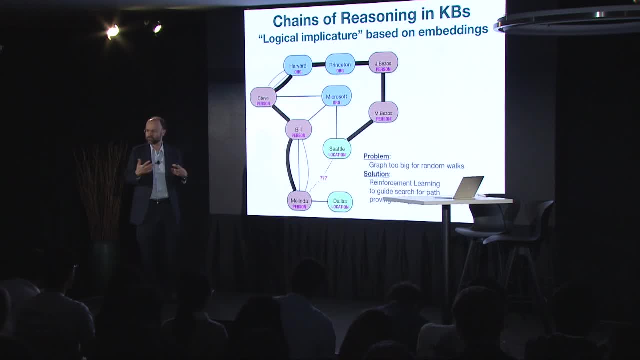 that are kind of just don't really carry any meaning at all, are just not relevant to the question that we're trying to ask, And in our original work we were just searching through the graph by doing random walks, but that's really not sufficient for the large scientific graphs. 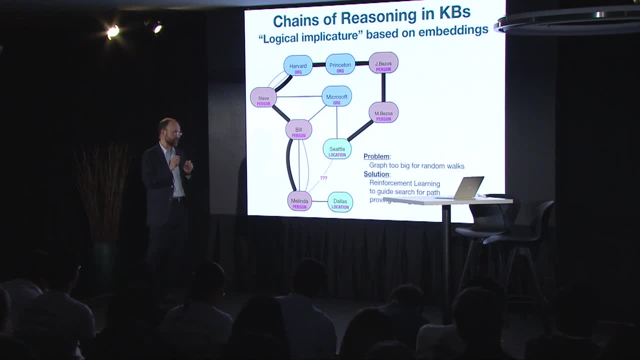 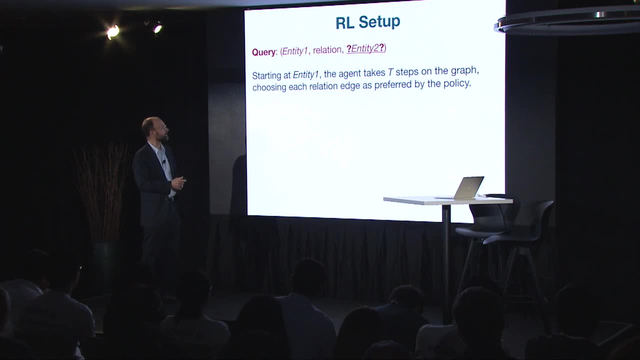 So we've been doing work on using reinforcement learning to guide the search for paths that prove the answer to the question that's being asked. So what does this look like? So it's afedular allows us to just start at some entity. At each entity there's a large 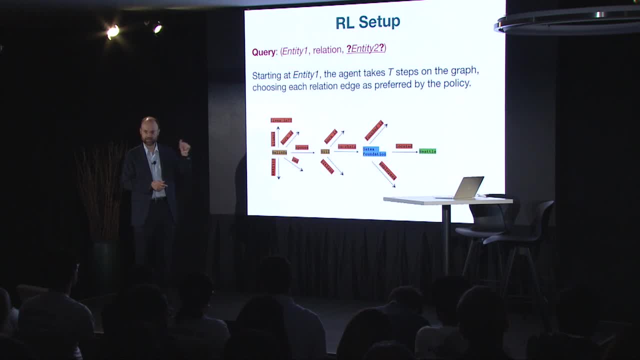 choice of different outgoing edges that we could follow in the graph. We make some choice. we continue to follow the graph until the model thinks that it's arrived at an answer. If the answer is correct, then we give the reasoning agent a reward. If it's. 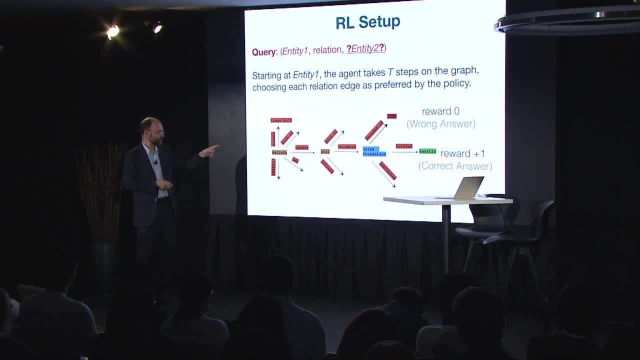 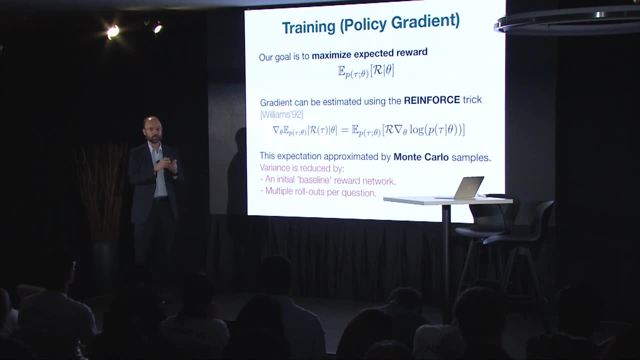 an incorrect answer. we give it no reward, we give it multiple chances to explore. Credit for write and wrong answers flows backwards through the graph And we can do some learning. gradient descent We are, you know. the training objective is to maximize expected reward. 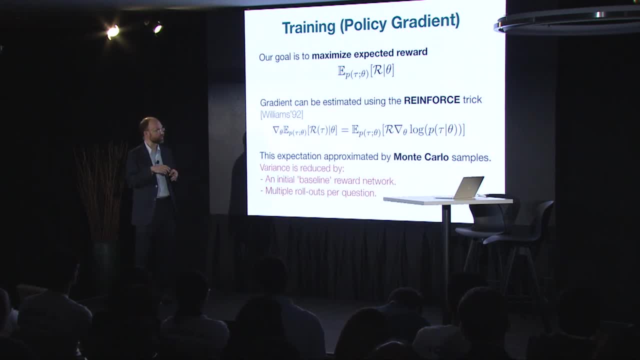 The choices to be made are discrete, and so we use the. we need to use the reinforce trick in order to get a smooth gradient out of a set of discrete choices, But this, together with some- you know- some various methods, like multiple rollouts per question, allows 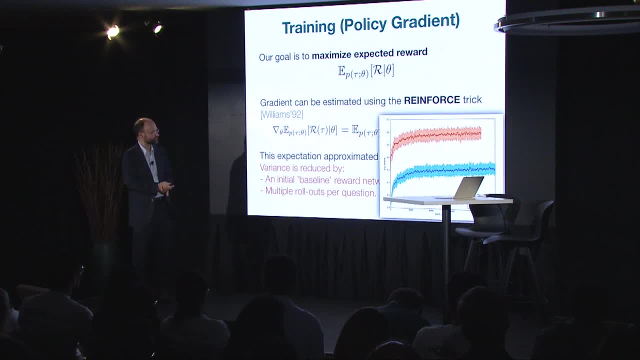 the system to converge and to reach, to reach very nice answers. Some other work that I'm not describing on a slide here, but I think for which there's a poster today, is using methods that are quite similar to this, even in a very large 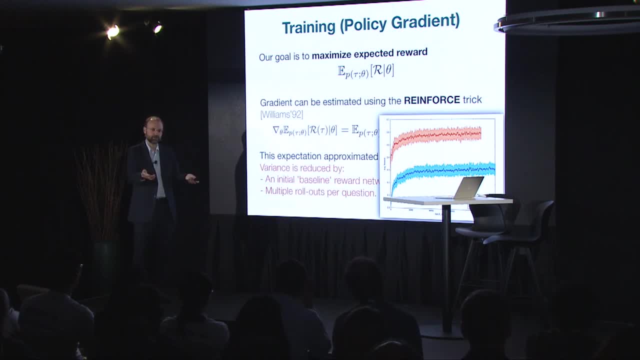 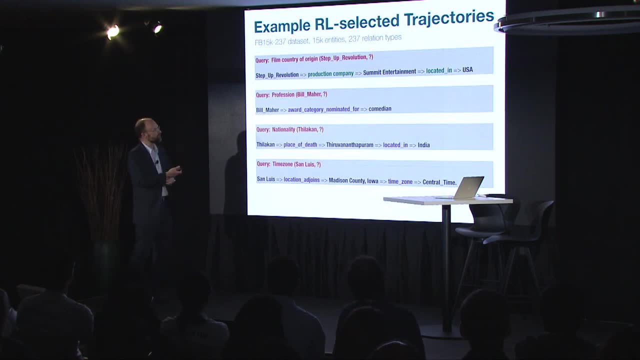 corpus, deciding even which paragraphs to read next in order to look for the answer to some question in some open-ended QA system. So to give you a sense of the kind of path that this reinforcement learning agent is able to find what it thinks of as most efficient. 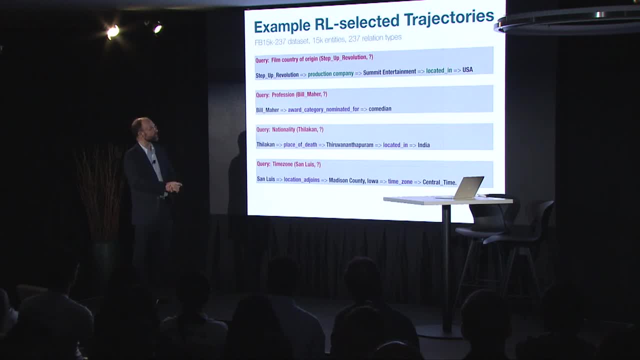 when asked say what's the country of origin for the film Step Up Revolution, it had no immediate evidence for what that was. but it jumps from the film to its production company, to where the production company was located, et cetera. 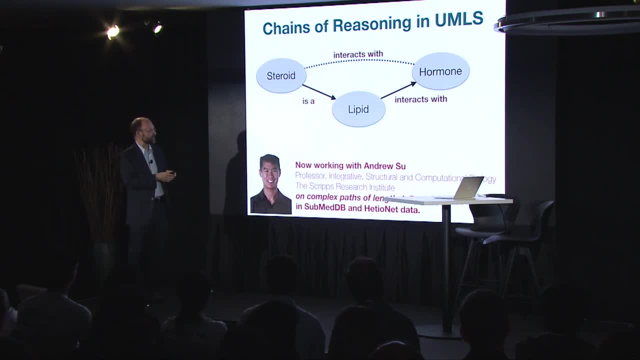 All right, So this is one. so here are some examples in general knowledge. We're now actually, you know, very interested in making work in biomedicine. We've been collaborating with Andrew Hsu at the Scripps Institute on applying this to to biomedical data, and we're looking 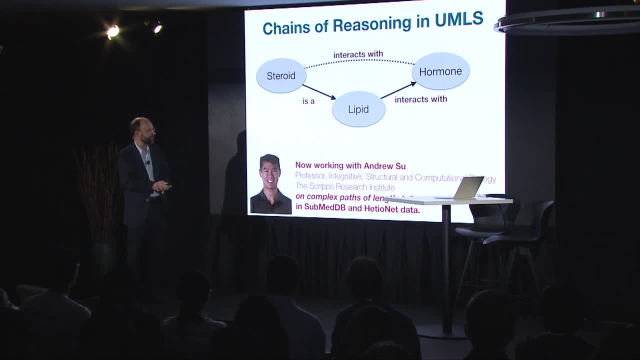 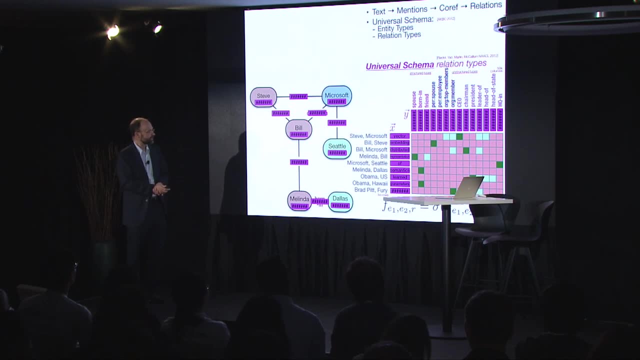 at much more complicated paths of longer length. And, yeah, we're excited about this work and would be very happy to find other collaborators, All right, All right, So I also find it interesting- let's see, how am I doing for time That you know these? 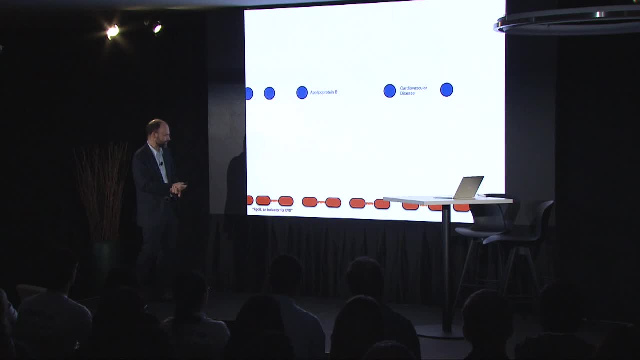 when there are many, many types. it's often the case. oh sorry, let me say something else first. So we, what we talked about so far fits into a worldview that I think somewhat like this At the bottom in orange. I'm trying to show some raw text here with entities in: 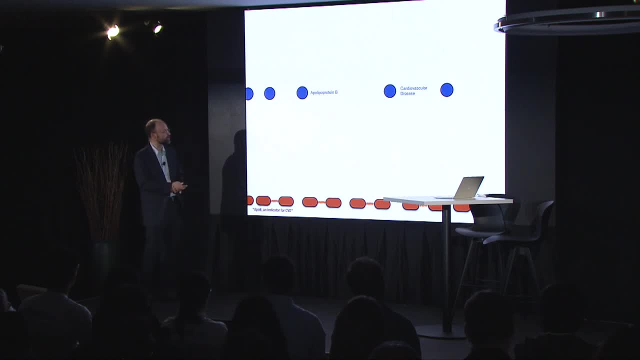 these ovals and the crayon mark is like some textual evidence of a relationship between them. And we use those, to you know, after linking them to some entities, to infer that well, I think there's something wrong with this. And then we use those to you know. 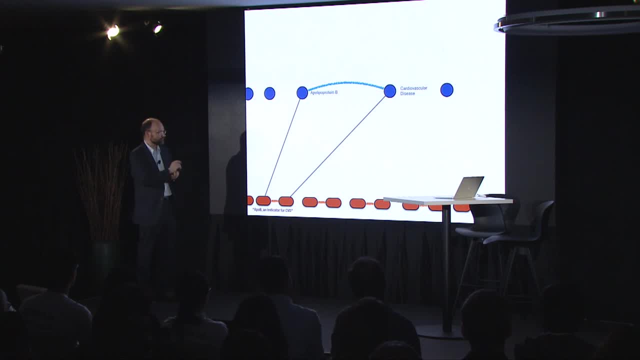 some relation between these entities and the knowledge base And this. this pretty much describes what we've been talking about so far in terms of raw evidence and the and the, the inferences we're making at the entity level, But I actually think that what we should 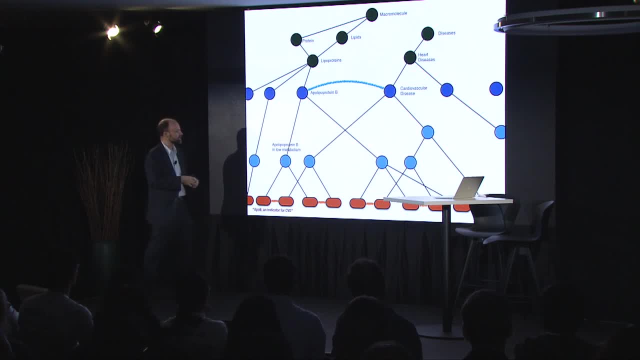 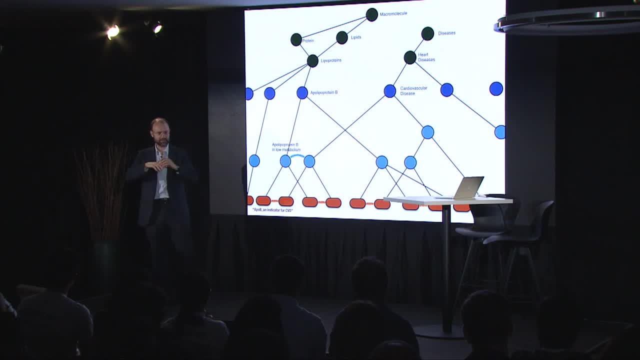 from illinois and as a president and past president, and and different relations were true of obama during these different stages. um, of course, we can also make some inferences at the entity level, but then there are also relations that can learn among types at even higher levels. 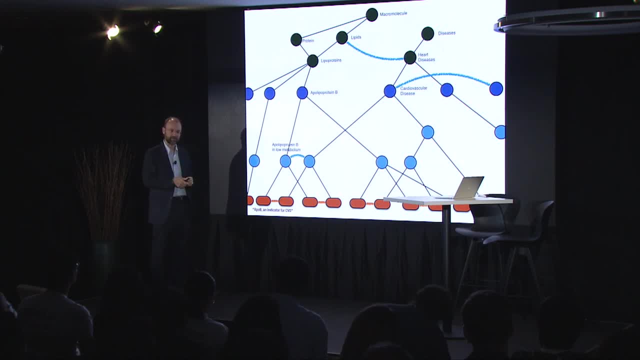 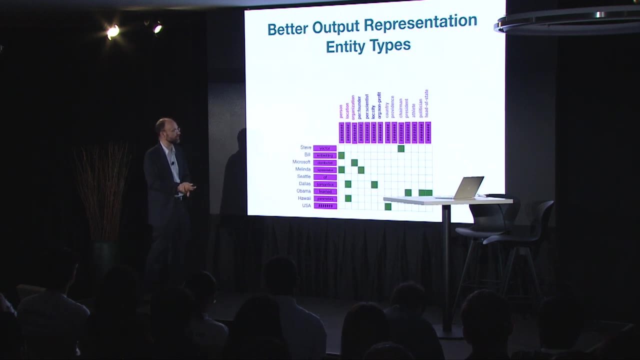 of abstraction, and i think about this as common sense, uh, um, relations among types, and so we'd really like to be reasoning throughout this graph and to reason about, um, hierarchies of concepts, uh, that exist in some hypernym relation throughout, and so this has us thinking quite a bit about. 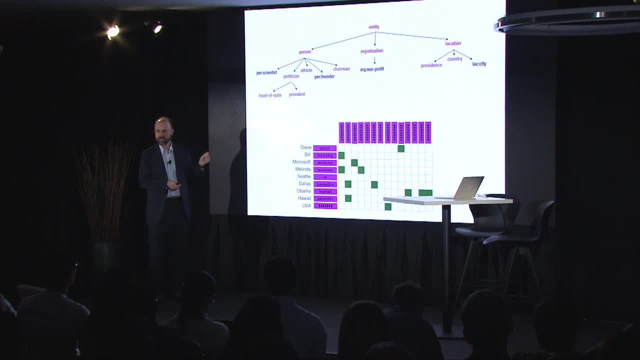 these types of entities and how it's often the case that they exist in hierarchies, and how can we use these taxonomies to help improve inference so we can work with various embedding methods that are that are aware of these, of these taxonomies, and use distance measures between vectors? 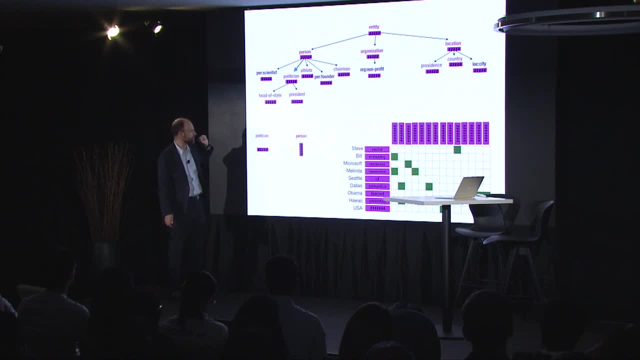 that that can be asymmetric to represent the asymmetric. is there a relationship there? so things like bilinear, maps that go through, instead of just a simple dot product through some uh, through some matrix in the middle, yield some asymmetry, symmetry also. if we have complex vectors, then those also have some. 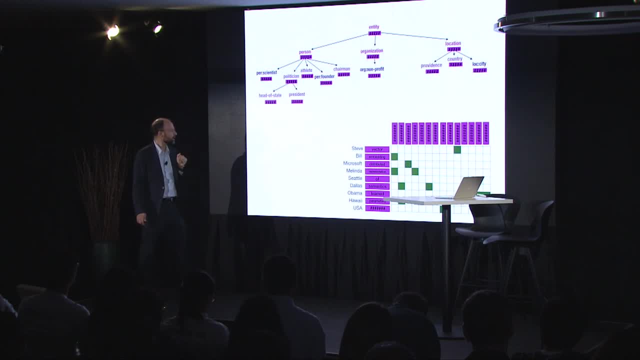 asymmetry. we can represent hierarchical relationships there as well. and then, um, when we see some textual mention, we can train some model that will create a vector for some textual mention. and uh, and then ask: well you know, does this vector have? the is a relationship with founder. 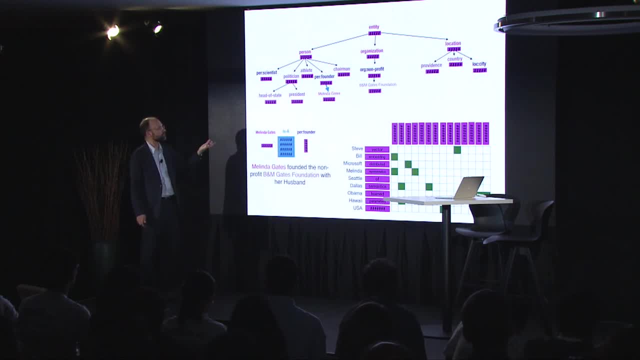 in order to answer questions um about types. but first of all we're going to look at some of the different types that exist in a hierarchy and, furthermore, also to leverage the hierarchy, because we also will have trained on pairs of entities, that pairs of types that fall into the hierarchy and um. so we've been looking at various 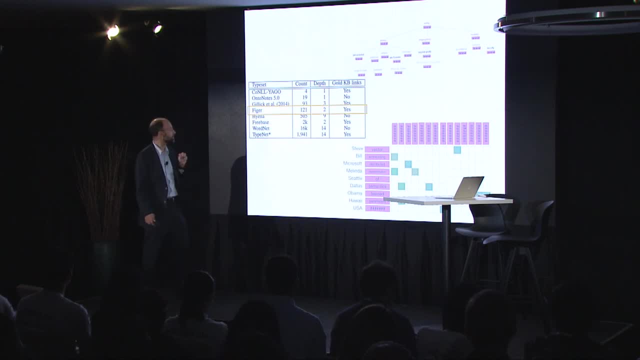 sources of data in which there are fine-grained types that exist in a hierarchy, and probably the most widely used data set for fine-grained types has been the figer data set with 120 types. but we wanted something much more substantial to reason in a much more fine-grained fashion, so we created 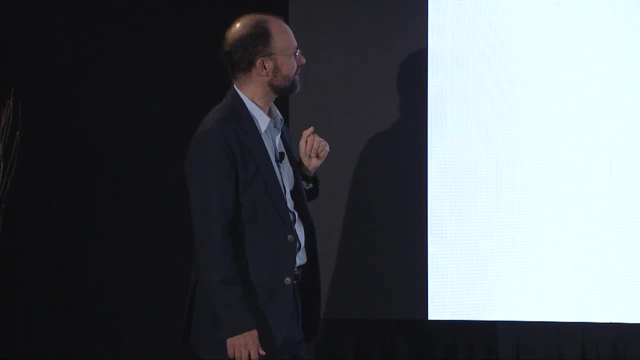 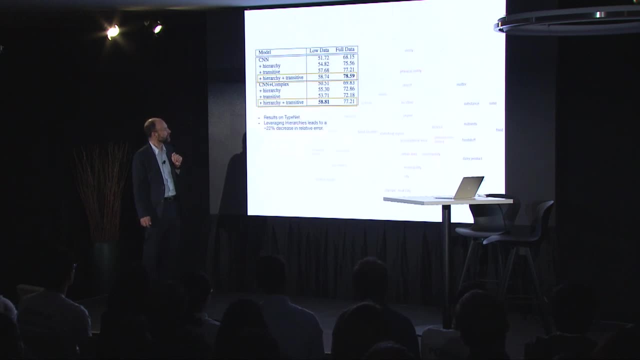 a new data set called typenet with almost 2 000 uh types in it. and what we find on this data set, um- this gives you some intuition for its level of granularity- um, and what its shape looks like, is that um leveraging the hierarchy yields to more than 20 percent decrease in relative error. 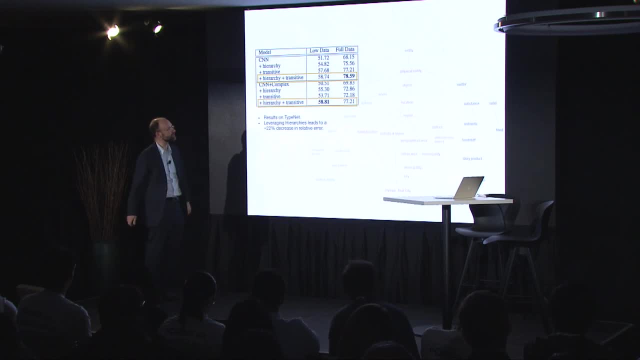 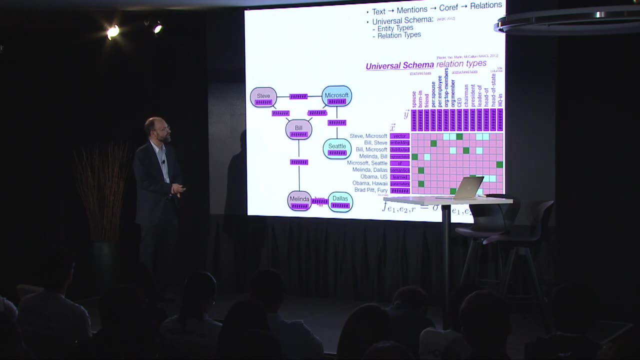 like here, going from 68 percent um up at the top to 78 uh percent, by using the fact that we know about. these things fall into a hierarchy, um, all right. so, lastly, we've been thinking further about other, more rich ways to represent um uh data sets, in the sense that, for instance, we could say that a data set is a reference. 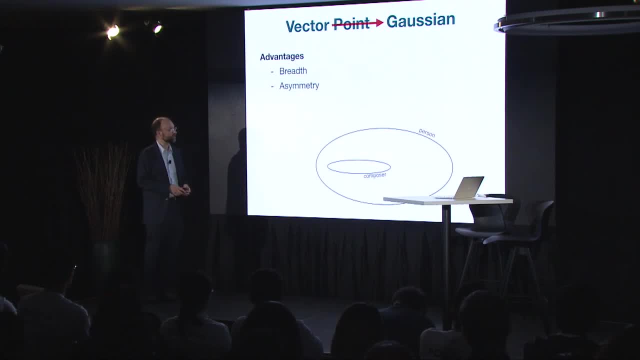 to a data set with more data in the setting space. then we get to kind of concentrate on the data set in a lot more detail and I think it's interesting to see that the way those data sets are represented by data sets we can see it's almost like a sort of a sort of a. 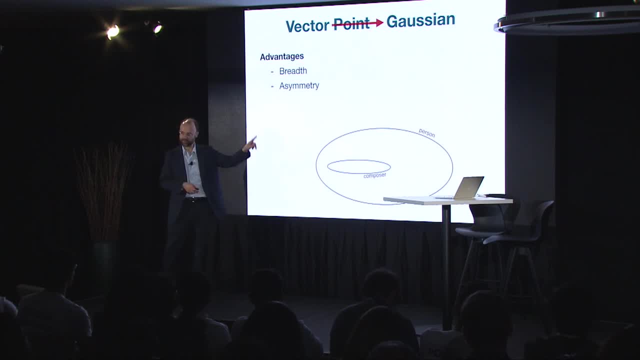 digital library and you have to think about the structure of a data set and you can see that the data set that is used and where the data is put is eight digit data sets. so this is pretty much on a that sits inside of it and that famous is a broad concept and we even just naturally learned that. 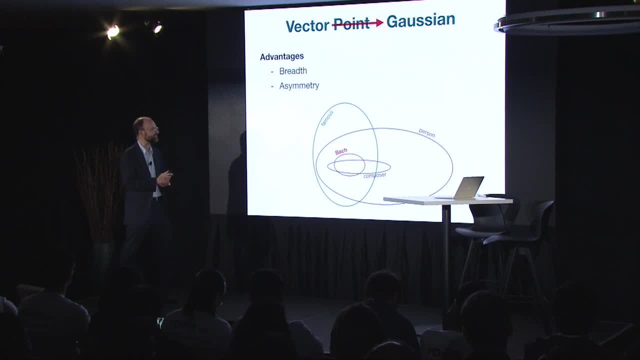 johann sebastian bach sits exactly at this intersection, which was nice to see, um, and so yeah, an embedding method that is able to capture variance is has some nice advantages, um, but gaussians in particular has some disadvantages, and one of them is that it's not closed under. 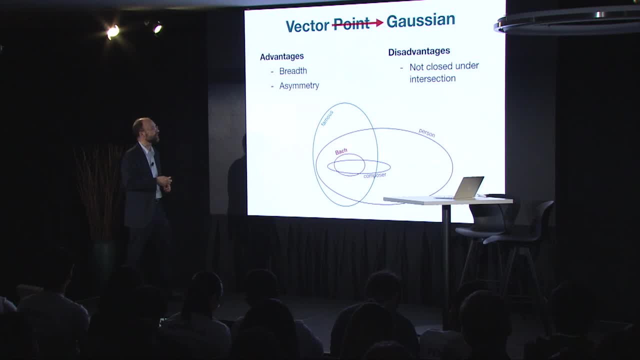 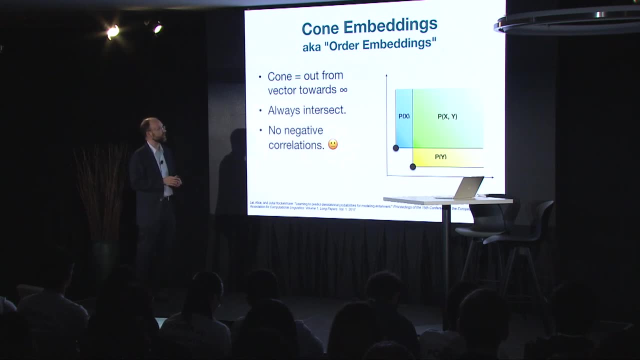 intersection, at the intersection of two gaussians, is not a gaussian, and so recently we um we've been looking at some other methods that do have this closed property. one of them is worked by others on order embeddings that uh defines. each um has, for you know, each concept of a vector, that's. 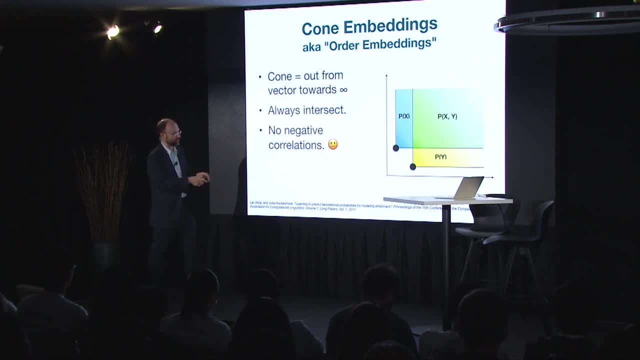 constrained to be non-negative and says that that vector actually defines a region of space that spreads out away from the origin, and um, and so the intersection between two concepts is exactly the point where they intersect here, as well as the intersection that spreads away from the origin, and so, um, this is closed intersection. 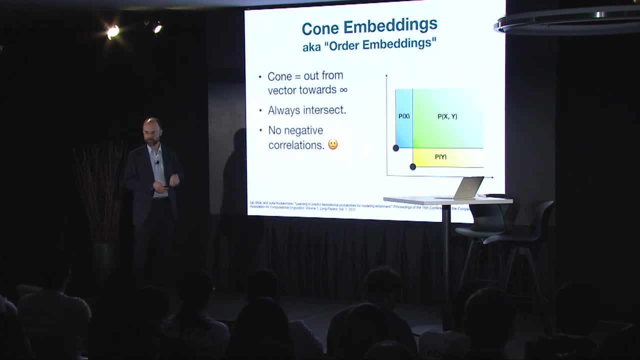 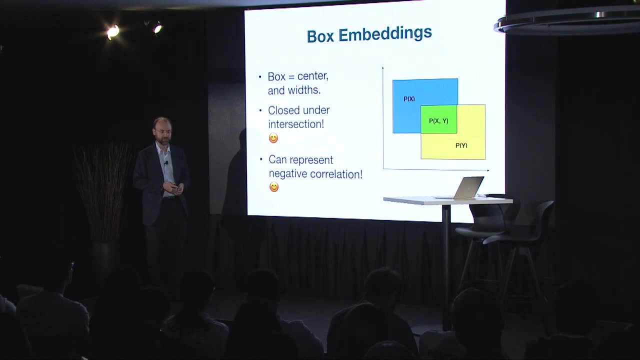 but the model mathematically is just not able to capture negative correlations, and so we just last year have an acl paper on this thing we call box embeddings, in which for each concept there is an n-dimensional box and the box is defined by a center and by its widths. 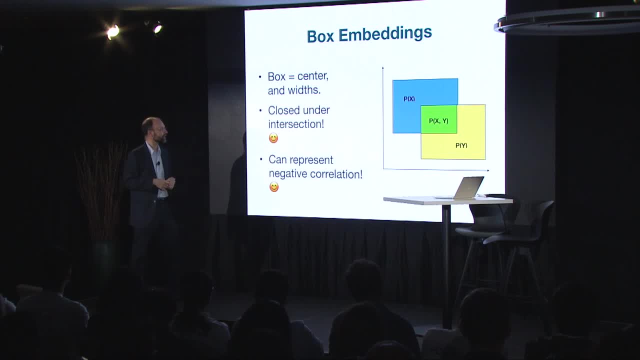 in each dimension. so it effectively just doubles the number of parameters. not that much if closed under intersection, because the intersection of two boxes is always another box and it can represent negative correlations. so you can think about these a lot like venn diagrams, right and the. you know the volume of the box will be proportional to its marginal. 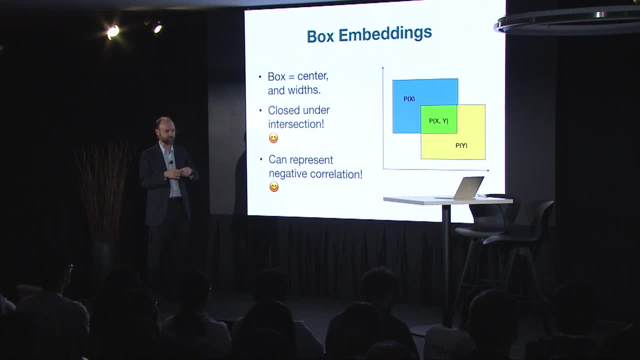 probability, the volume of intersections, uh can be used to calculate conditional probabilities and we can also condition on multiple other boxes, looking at the intersection of all of them, to answer really quite complicated questions about conditions. on this evidence, what do we believe about the probability that certain other things are true? in fact, we're even investigating these. 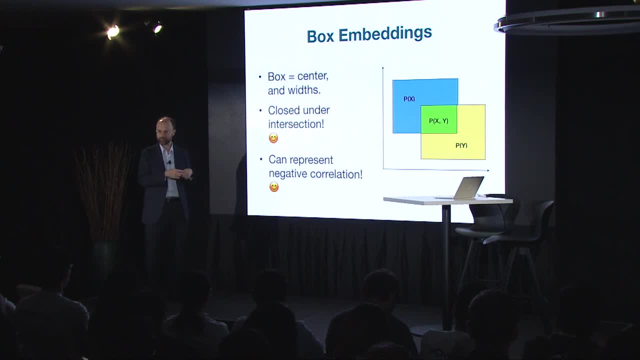 as a whole cloth alternative to graphical models. um, i think there are some things that these definitely will do worse than graphical models, but something that's they will do better than graphical models, and that they can efficiently do inference on, say, hundreds of thousands of variables and answer probabilistic questions about them in ways that 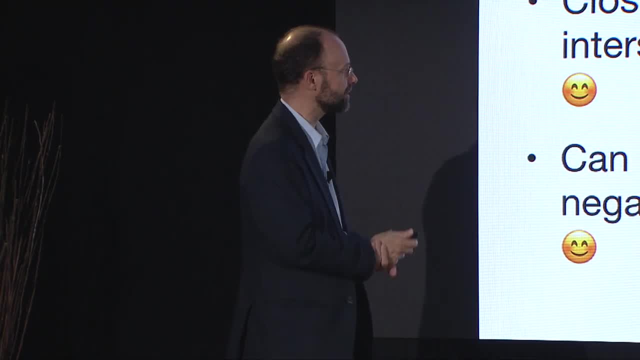 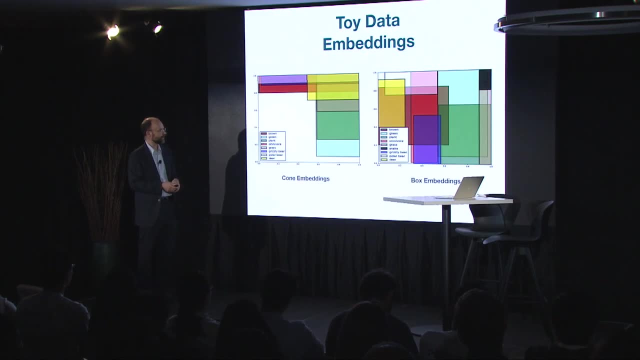 don't rely on there being sparsity among the dependencies among them. So, on some toy data that we just created by hand for the sake of just understanding what was going on in the model, what we find is that, in comparison with order embeddings, our model is able to, you know, learn. 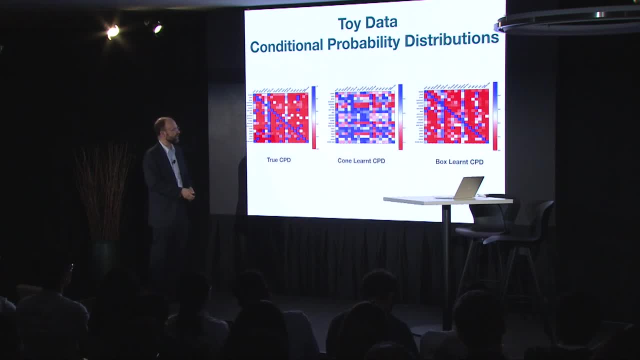 sensible boxes with sensible overlaps and to use the space well and, in fact, fit it much better. So here's the true conditional probability table that was part of our training data order embeddings was not able to match that very well at all, but our boxes were able to match it. 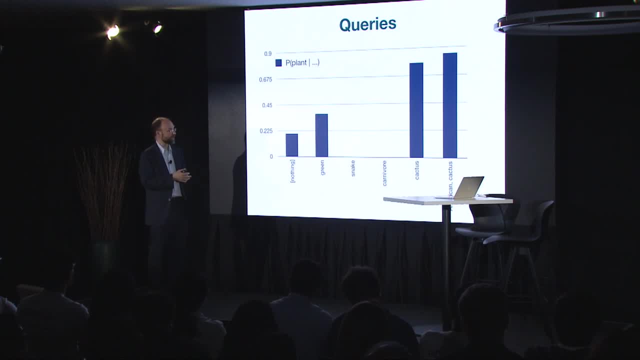 quite well, and we can see that it's also able to represent negative embedding, so negative correlations. So here we're asking: well, what's the probability of being a plant? conditioned on nothing, just the prior is this. but conditioned on being green, your probability being a plant goes up. 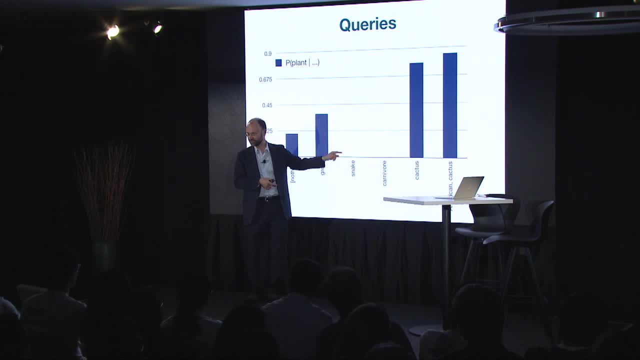 and so on. So here we're asking: well, what's the probability of being a plant, conditioned on what's the probability of being a plant given that you're a snake? Well, it's zero. that's a negative correlation, and that's what order embeddings would not have been able to represent. 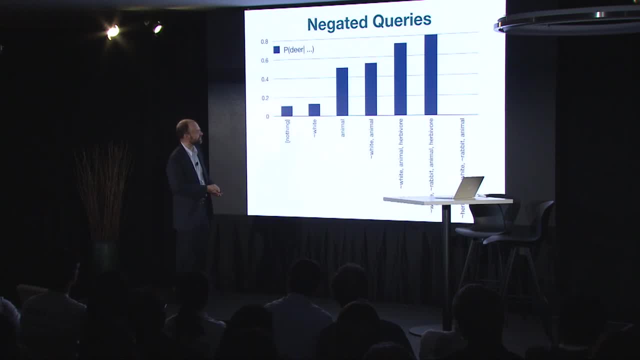 at all, And even with multiple queries, we can represent things like this: So what's your probability of being a deer, given that you're not white, and so on? All right, But what really matters, and what's more interesting to me, is something like this in which we are operating. 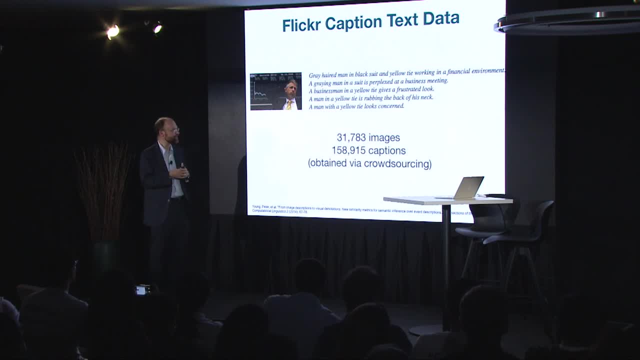 on arbitrary pieces of text and doing what I really think of as a kind of common sense reasoning. So there's a Flickr data set in which we're going to not concern ourselves with the images, but just the textual captions that people put on these images, And it's a large collection. 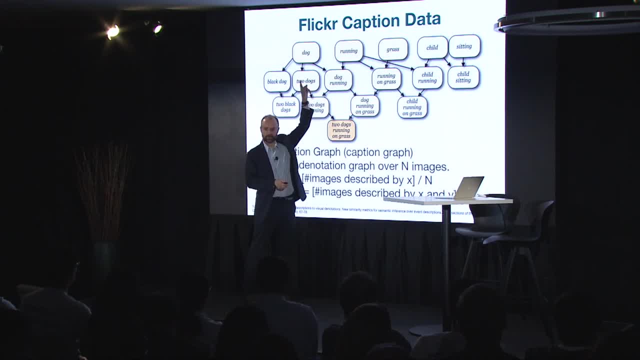 And for each caption we're going to use a parser to break it down into smaller pieces so that we can get both sort of fine-grained pieces of text and coarse-grained pieces of text that describe the image, And then we can calculate conditional probabilities right by. you know what I'm. 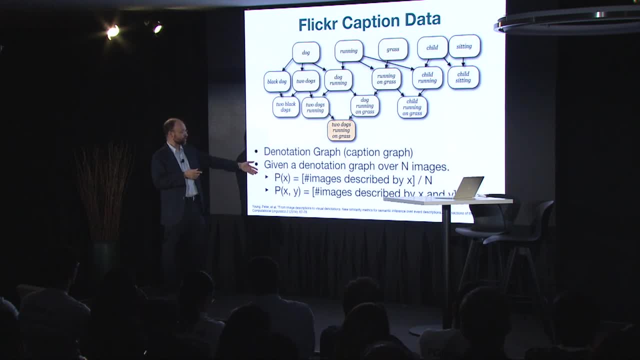 saying, First of all, it's the marginal probability of finding an image of a dog. Well, you know how many images were labeled with the dog somewhere, even if the original caption was something much larger. There's the smaller case here. We can also ask about joint probabilities. 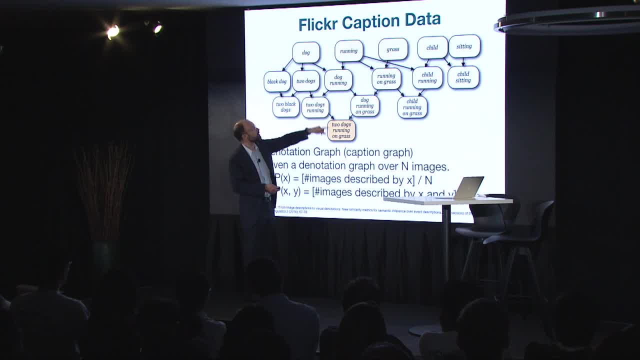 What's the probability of seeing both dog and grass together? Well, here's one, And we can do that by counting the number of images in which dog appeared at all or which grass appeared at all. And what we're going to do on our model is take an LSTM that's going to run over arbitrary. 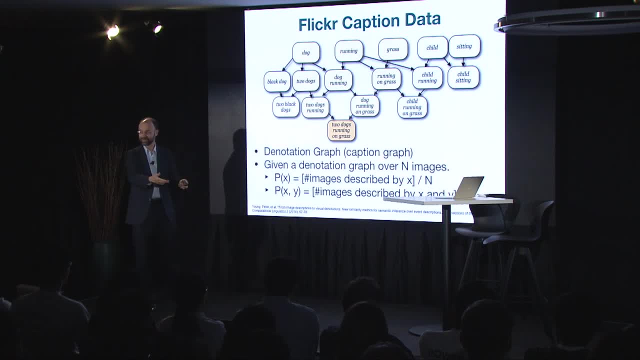 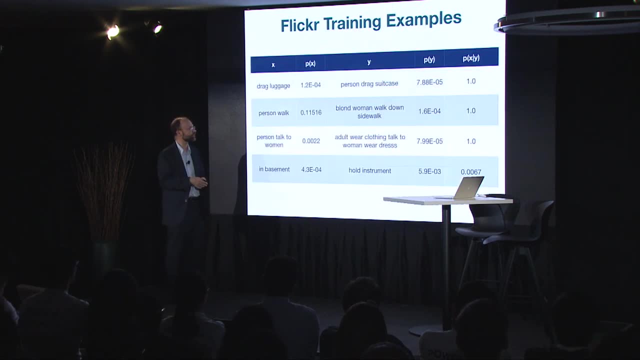 length sequences of text. LSTM is going to output a box And then we can look at overlaps between these boxes, to ask conditional probability, what I think of as sort of common-sense type questions. So here are some simple examples. If you observe a caption like a person drags a suitcase, what's the probability? 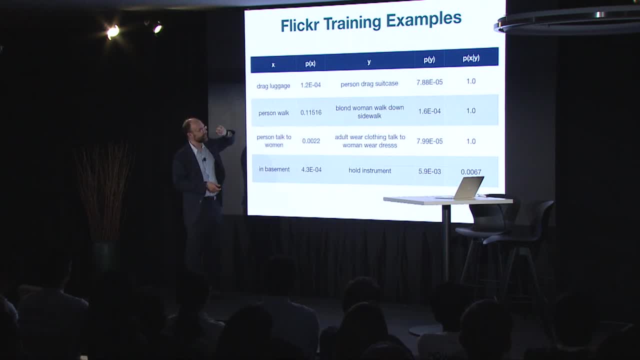 that you would say that implies that luggage is being dragged. Well, that's probability one. If you're told, well, there's someone holding an instrument, what's the probability that you're in the basement? Well, that's probability two. 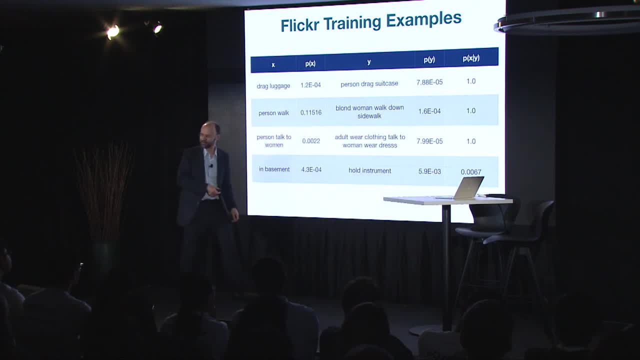 And it's low. It's not zero, but it's low, And I would say that that represents a kind of common sense And we're now applying this to scientific text. One of our goals is to capture scientific common sense And this yielded a new state of the art on Flickr And there's some new results about. 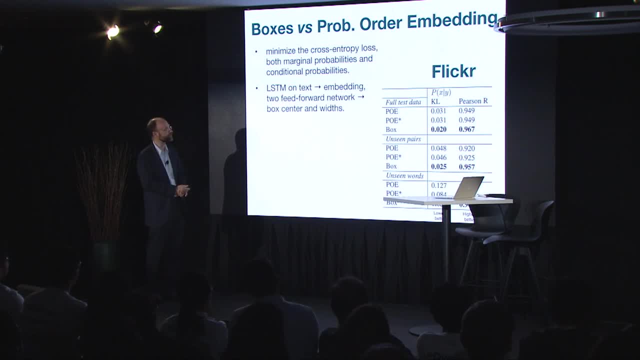 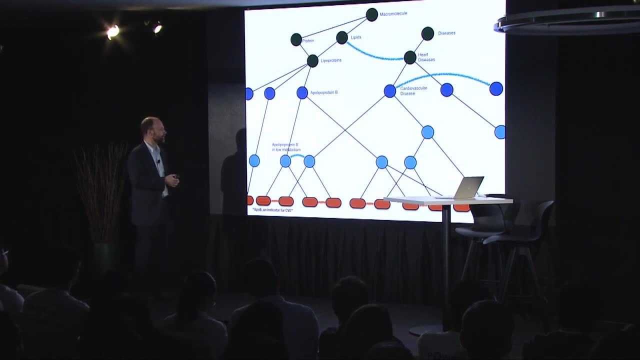 this, which you can also see in the poster by Lorraine Lee, one of my students who is here today. All right, So what we really want to be doing in the future is to be reasoning about large graphs like this, with many entities at the subentity level and at the type level as well, represent their mutual 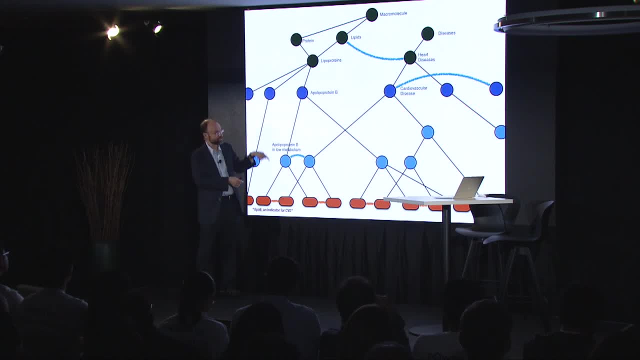 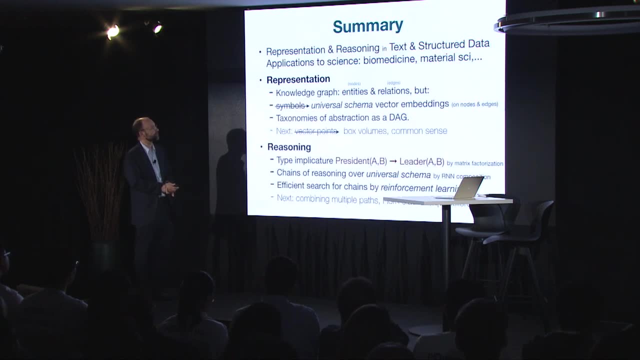 implicature with boxes and reasoning through chains. in this graph, various levels of abstraction throughout, And this is the research path that we're on. We've talked about representation and reasoning in text data using, instead of symbols, universal schema, vector embeddings and. 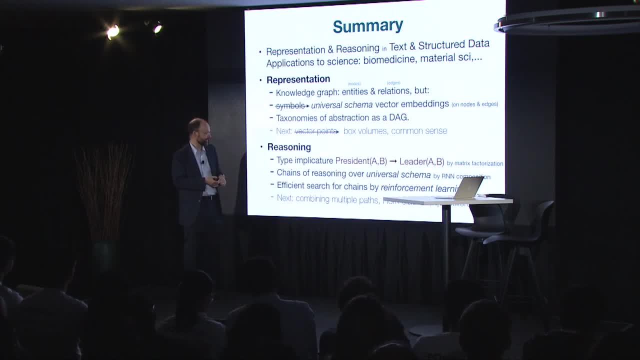 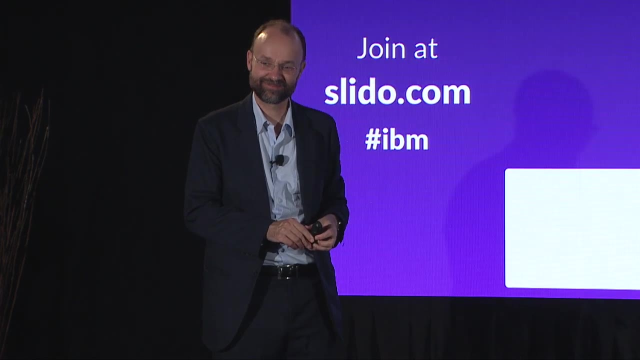 representing taxonomies by using box volumes. We've talked about chains of numbers, We've talked about lines of reasoning And with that, I'd be happy to answer your questions. Thank you, Let's see. So how does this work? Oh, they're there, Sorry, Thank you, Okay, Thank you With scientific. 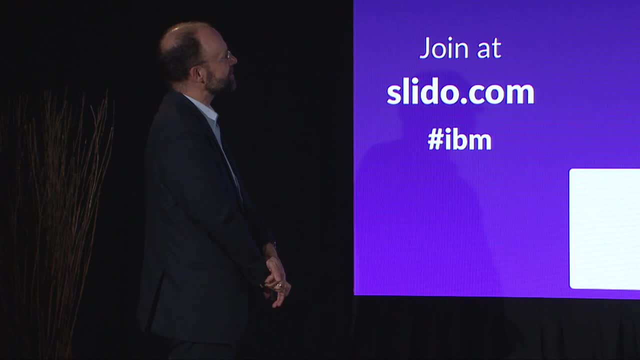 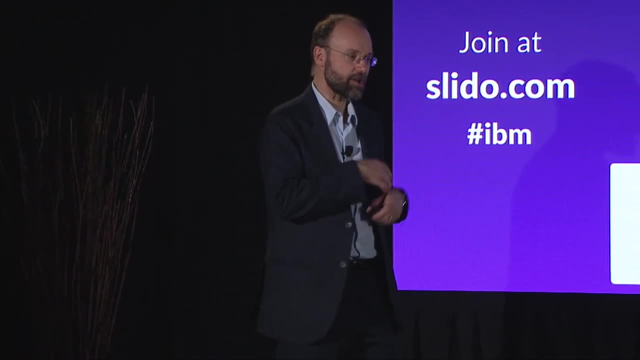 papers. what happens when there are contradictory relations that are extracted and added to the graph? Okay, Yeah, Wonderful. So in the original work we take all the text as training data and, as so often happens in machine learning, we both in a way assume that the training data is true. 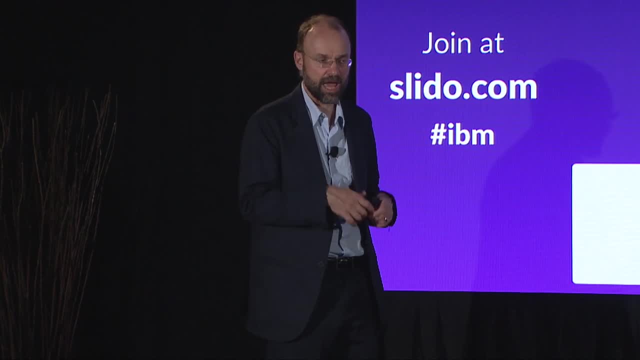 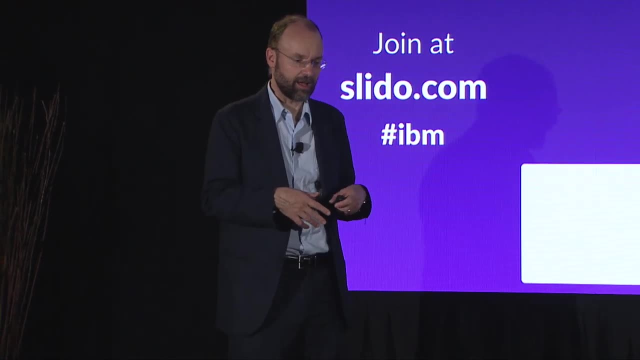 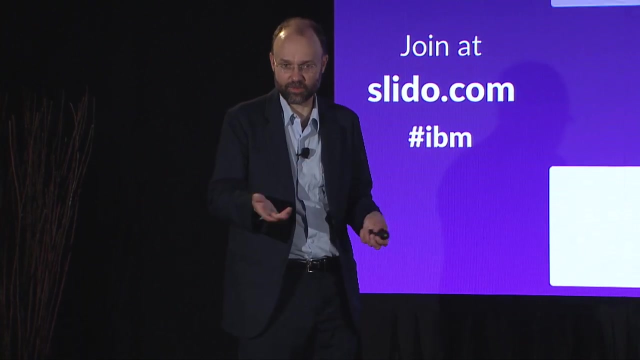 but the training is robust to noise in that data. When asked questions about what might be true again, as is often the case in machine learning, we'll rely on most statements in the training data having been true and we'll answer what the majority opinion was in the original raw training data In the 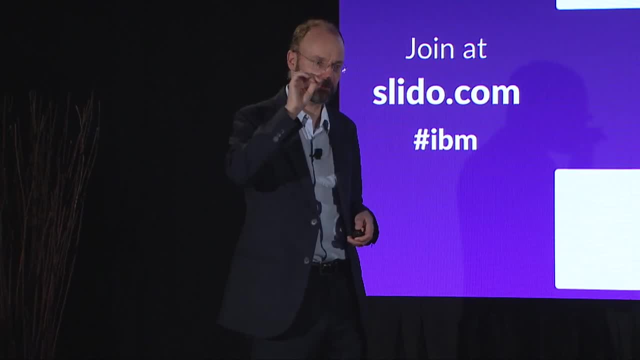 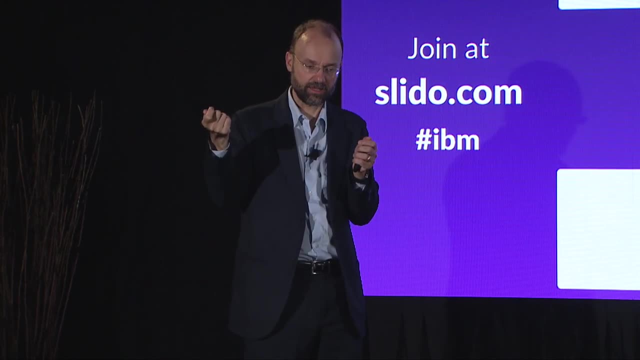 chains of reasoning work. so far, we've been able to do a lot of things. We've been able to do a lot of things And so far, what we do is we look for many possible paths that could provide, you know, evidence of a positive answer to something and you know, zero in or pay attention to that one path. 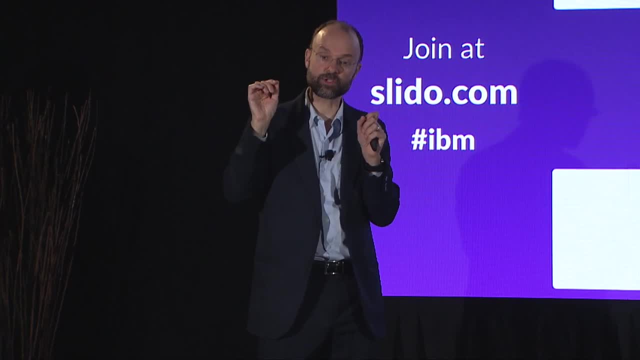 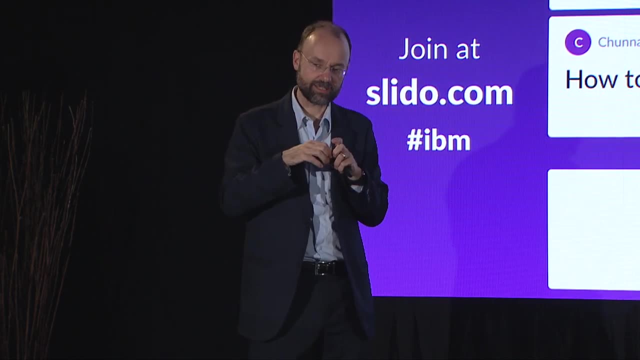 and then ask: is the strength of that evidence above threshold for us to say yes? And I think this was a reasonable way to start. but what we're considering doing next, which I think is necessary, is also to look for negative evidence, like: look for the path that would make us most strongly say: